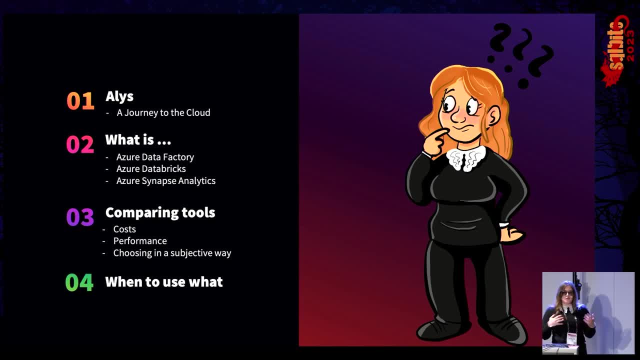 she is going to make her journey to the cloud. Of course, some of you might not yet have seen any of these tools, So it would be nice if we kind of already knew what Azure Data Factory, Azure Databricks and Azure Synapse Analytics was. So we're going to talk about 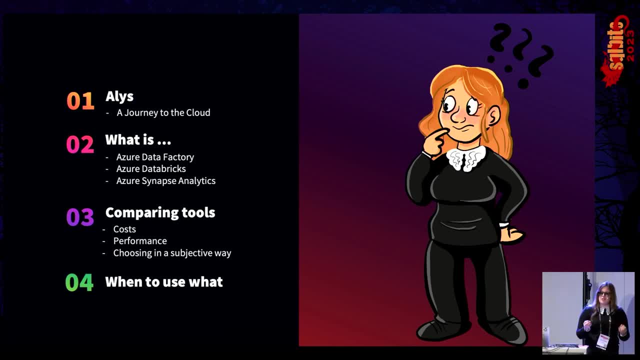 that next, In the end, we want to make a comparison, to compare these tools right. So we're not only going to look at functionality, but we're also going to look at cost, at performance And lastly, maybe one of the most important things- is to make a decision in a subjective 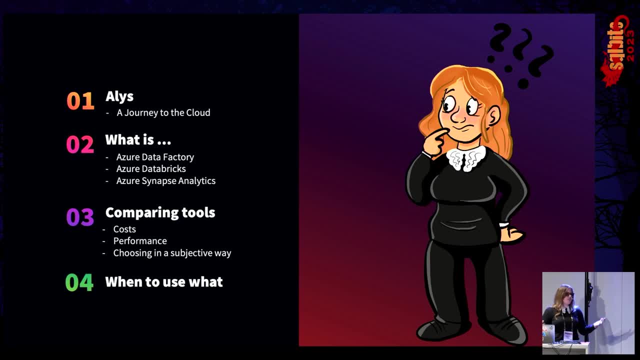 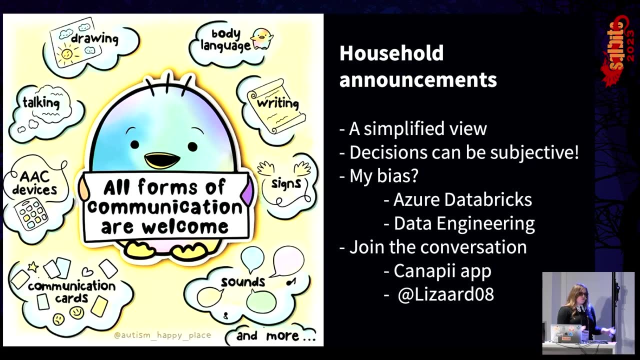 way. We're going to talk about that too. In the end, of course, we have to reach our conclusion right- When to use what. But before we start, let me just give you a little bit of background information. So 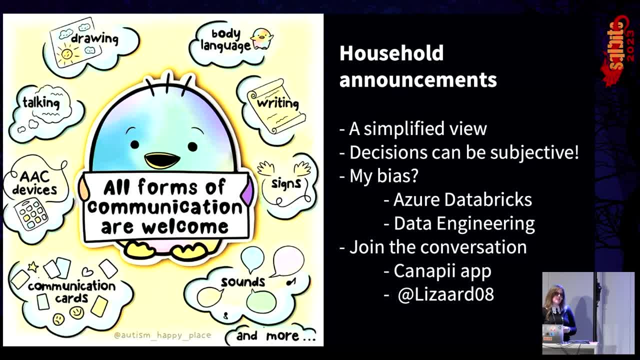 let's start. I want to make some household announcements. At this moment, we only have like 15 minutes, right, So that's crazy short. It's going to be a simplified view. Just to get to know one of these tools would already be a course that takes multiple days. I don't. 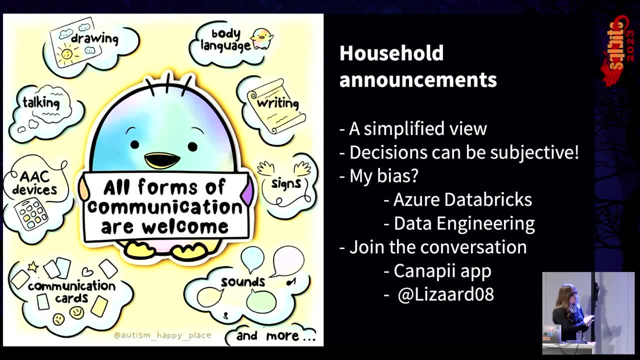 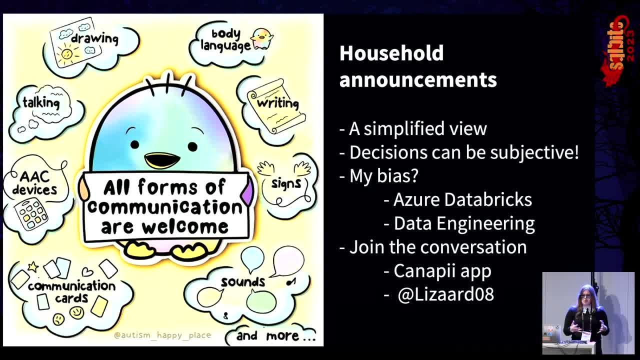 that's the tool that's always near and dear to my heart. At this moment I use very often as a data vector, so this is also a tool I'm a little bit more acquainted with. The point of view that I have is going to be data engineering, So for data signs use. 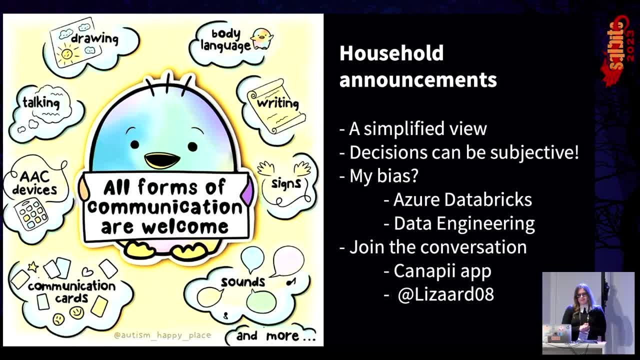 cases, my knowledge might be a bit limited compared to others that have that specialty. In the end, you're more than welcome to join the conversation. As you might have already noticed, I'm wearing my glasses today. I'm wearing the aud�s glasses when I longing for. 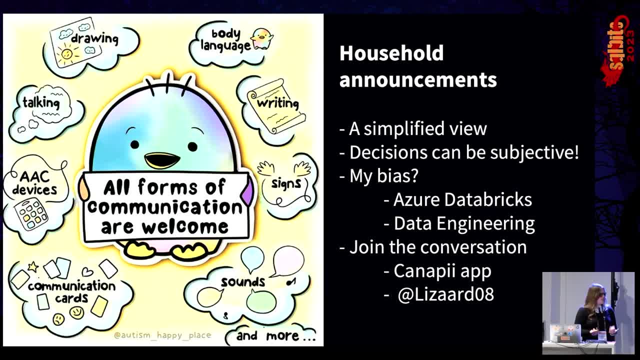 today is because I'm autistic and I have ADHD, so the lights are very bright as an input for me. So if you ever, during this talk, might feel a bit anxious or you want to stand, I'm not going to penalize you for it. I already see some people standing in the back that. 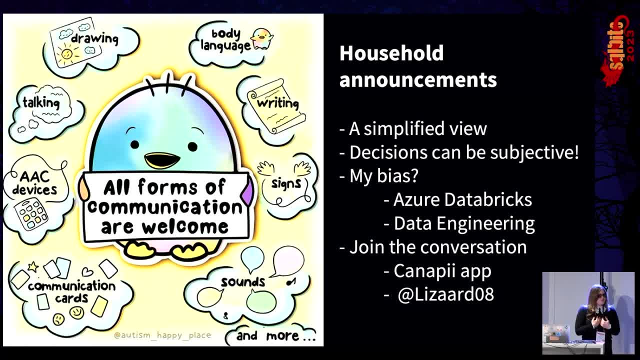 might be due to choice or might not be due to choice. For me that's totally fine. If you want to interrupt me during my talk to ask a question, you're more than welcome to raise your hand and just ask a question. If we go over time, though, I will let you know. 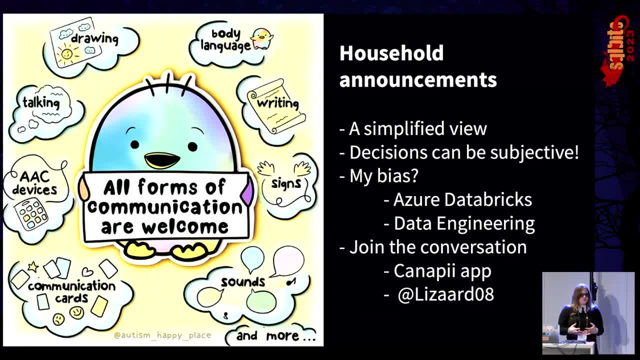 to keep it for the end, But if that feels uncomfortable to you, then you're also more than welcome, of course, to ask a question via the app. I think I'll see them coming in here, but if I forget about it, I guess somebody in the back will raise their hand. 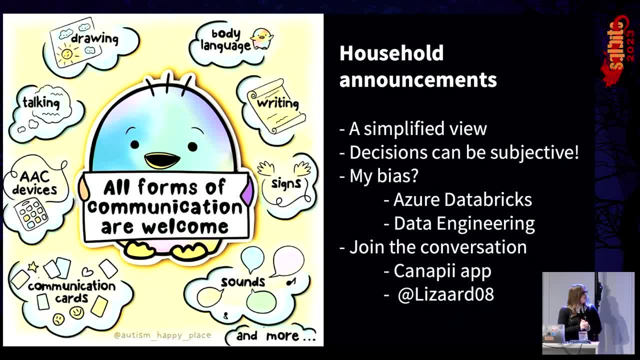 and be like: hey, Lisa, you're forgetting something In the end. if you wanted to ask a question but didn't feel comfortable to do it today, always feel free to reach out. via the soaps. I did bring some fidget toys, So if you want to have a fidget toy, just raise your hand. 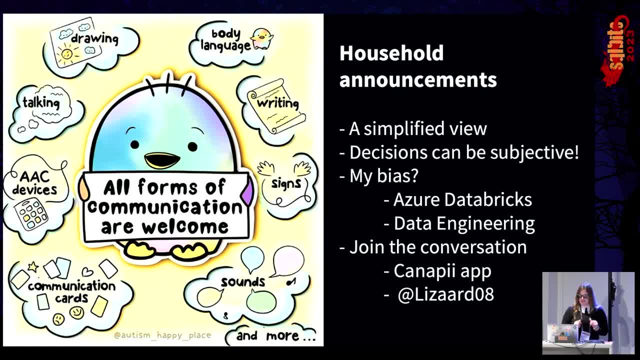 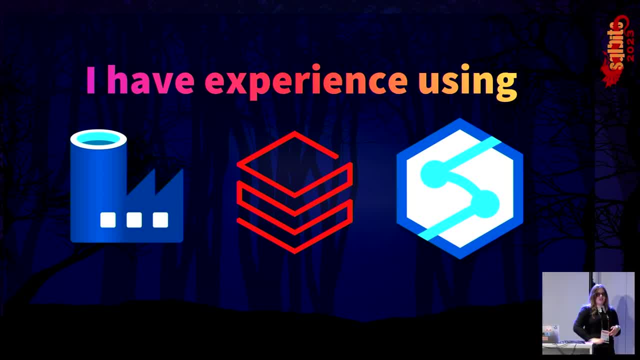 and I'll throw it your way, hopefully the right way, Or just come and grab it. That's totally fine. So to start, who has experience using Azure Data Factory? All right, All right. What about Databricks? Quite a technical crew here. Synapse Analytics, Somebody already? 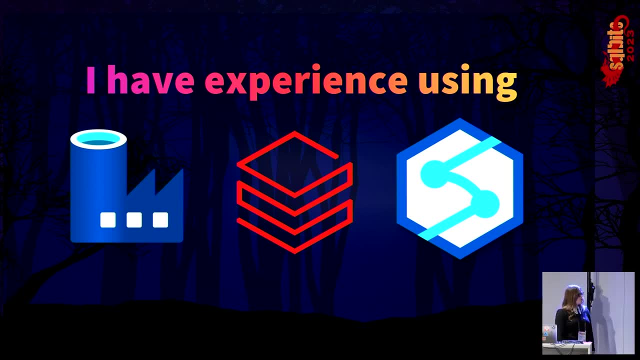 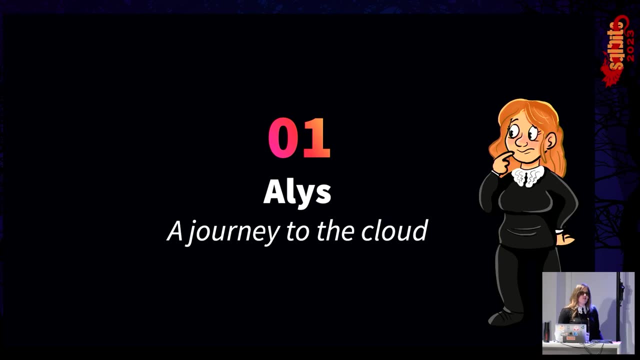 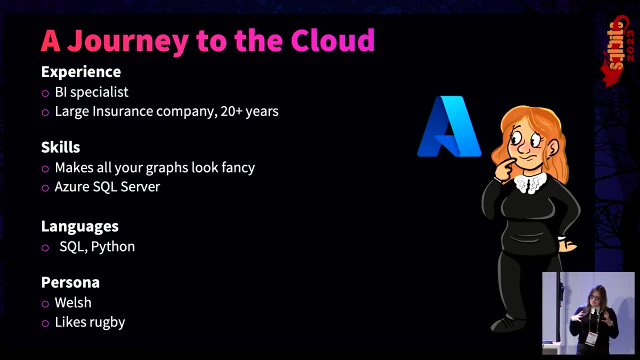 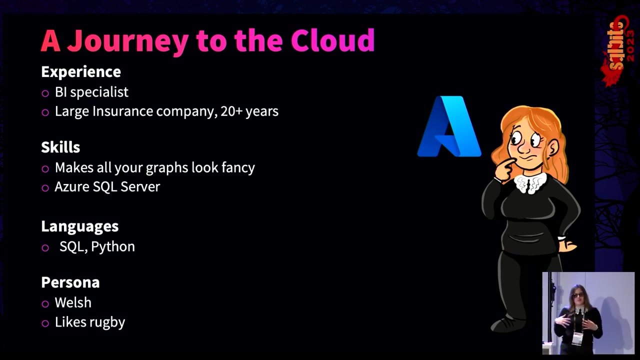 kept raising their hands like, yeah, Pretty cool, Right, But Alice has never heard about these tools and she needs to make a journey to the cloud. So how are we going to do that? Who is Alice? Just as a quick story, I usually present this in the Netherlands and I use a guy and his name is Henk, So Henk. 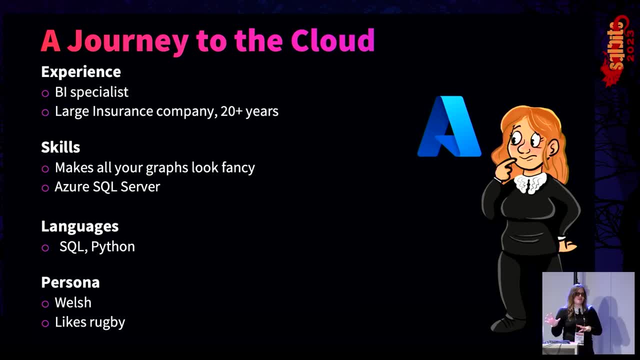 is basically the most random, like most often used Dutch name ever. So I went on the Internet. I've never been to work, I've never been to work, I've never been to work, I've never been to Wales, just to confess. So I Googled like what is the most common Welsh name? And 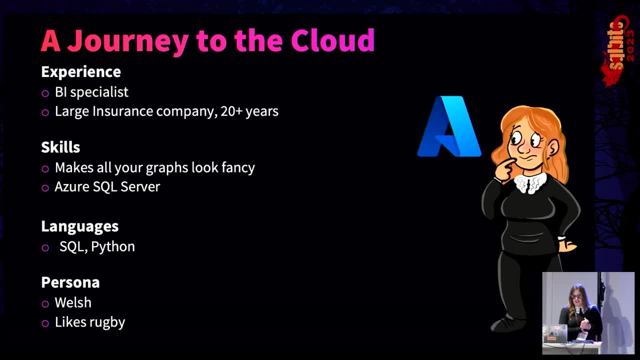 the first thing that popped up was Alice, So I named her Alice, And Alice is a BI specialist. She's been working for this large insurance company for over 20 years. I mean, wow, She has so much experience, Her skills. She can make all of your graphs look super fancy. 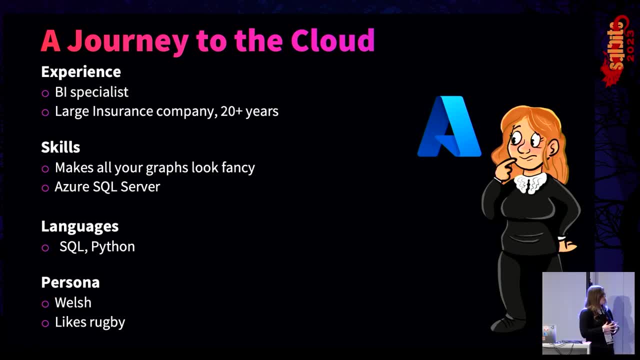 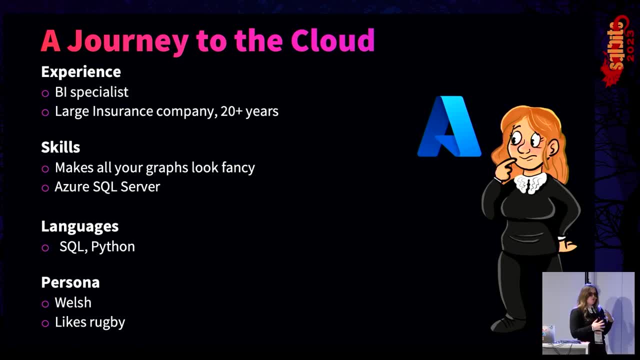 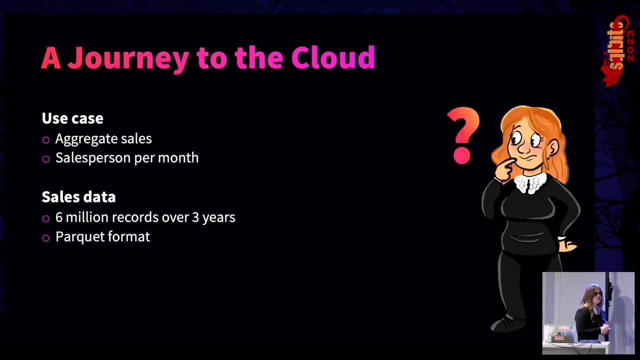 know, I don't know, I don't know anything about the right thing to do. Okay, Exactly, Ah, That's great. from month to month, It's an easy question, right? What salespeople did the best job? Who sold the most things? Just quite a lot of sales data. I think this is a very big 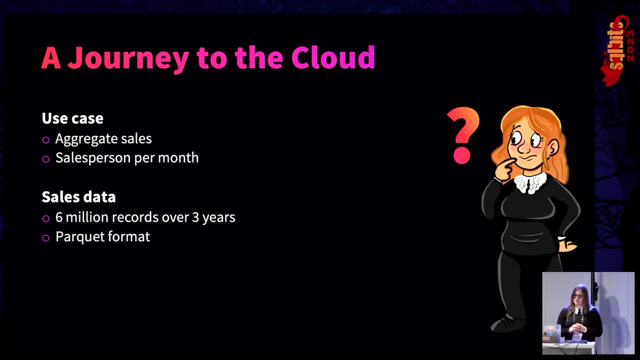 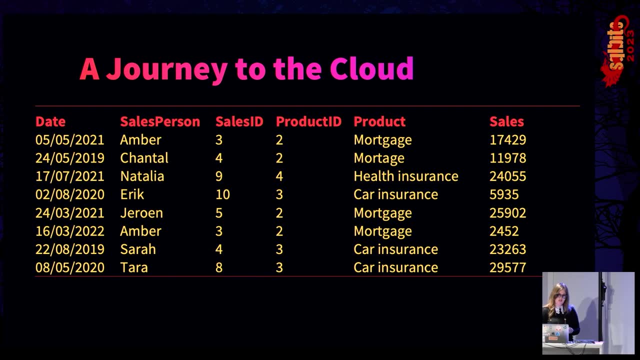 company, right, About 6 million records over three years. Well, we're just going to store that in a parquet format, right, That's quite run of the mill. But what does this data look like? Well, I hope this is visible for everybody. but just to go through it real quick, we have: 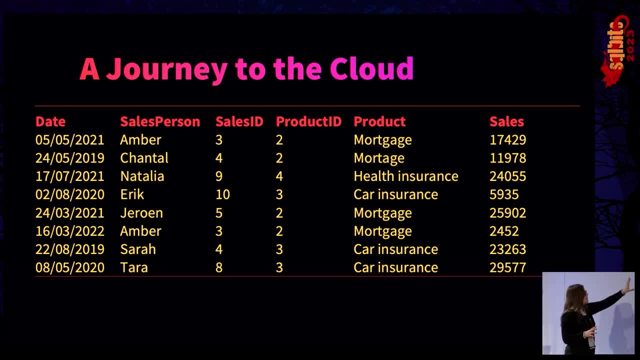 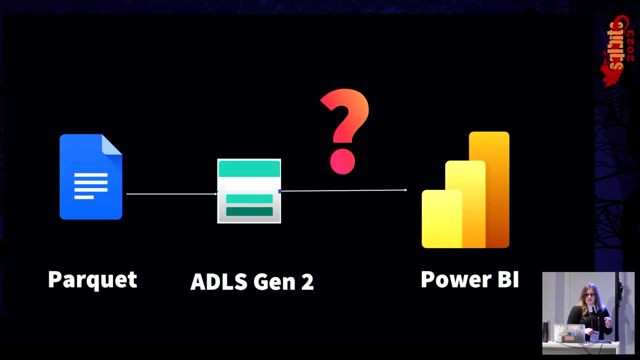 a date on which the sale is made. then we have the salesperson that did it, an ID for the sales and the product, then the product and the sales amount. So it's quite a diverse company. I would say Some mortgages, health insurance, whatnot? So what do we know? We? 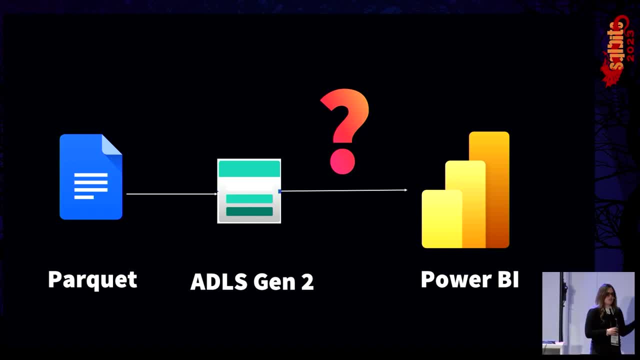 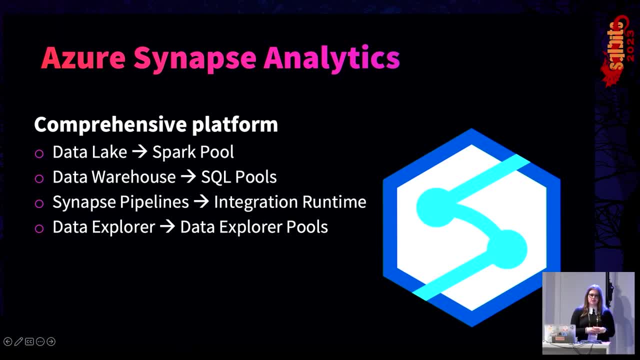 in a data lake. So what's quite run of the mill on Azure is to just store it. you know, If you want to have more data warehouse, you can use SQL pools, either dedicated or serverless. of course, Synapse pipelines, that's basically. well, basically a one-on-one copy of Azure Data. 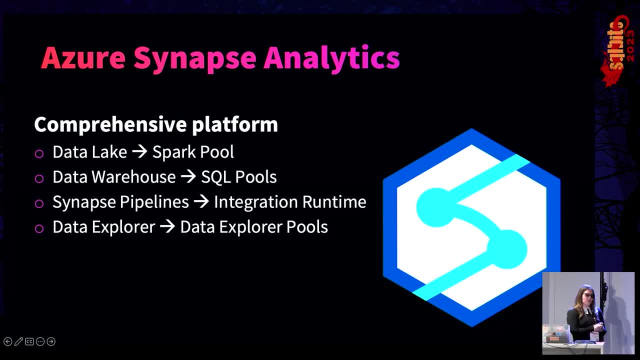 Factory. So I mean, why not take account of the powers of Azure Data Factory? right, We just call it Azure Synapse Pipelines. As we already know, these pipelines, the computational power comes from the integration runtime. If you want to create more, let's say telemetry or log data, then now we have that data explorer. 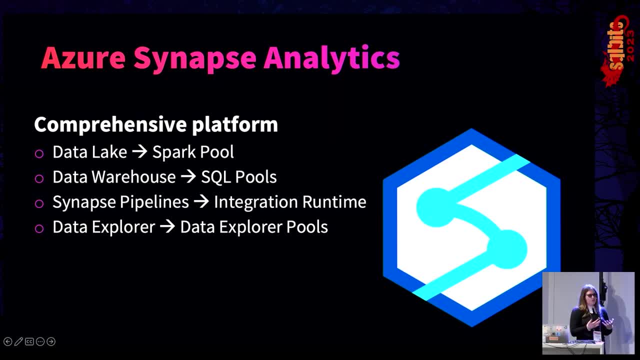 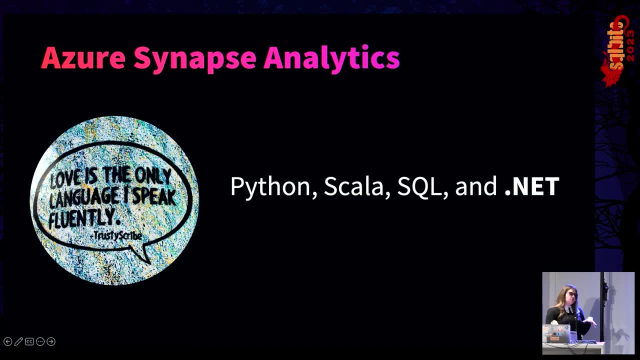 in preview for us. It's quite a cool tool And the computational power comes from the data explorer pools. So what languages do we have here? And this is more specifically to Spark, because obviously, if you do the data explorer pools, it's KQL. 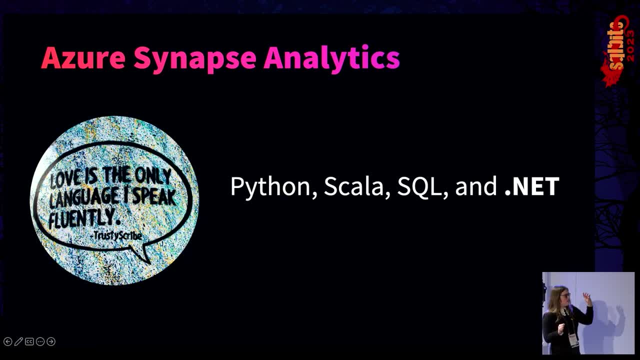 Some people really like that. I just can't, But okay. So the languages that we have is Python, Scala, SQL and NET. So if your specialty is in Java, go with Databricks. If your specialty is in NET, make sure to go with Synapse Analytics. 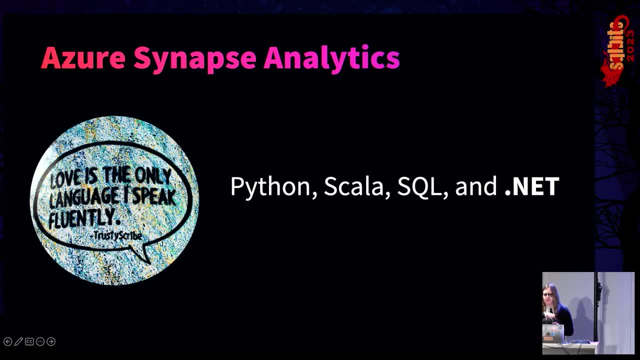 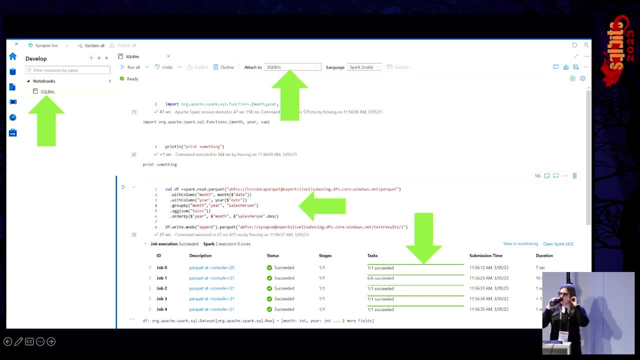 That's just how it is All right, But what does this notebook look like? Okay, So it's pretty much like a Jupyter Notebooks kind of environment, and much the same as what we see with Databricks, right? So I have my notebook here that I created in the left arrow. 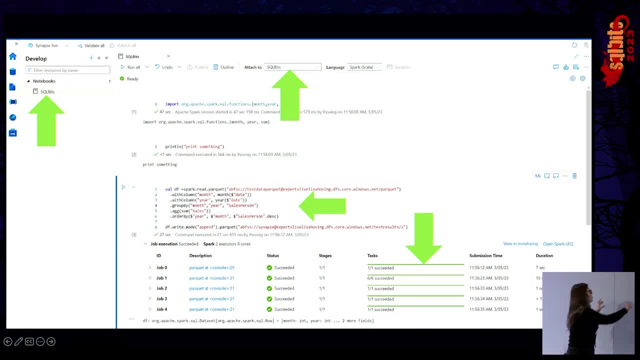 Then I have a cluster called SQL bits. Okay, Don't tell anybody. I said that It's the ADHD I swear. So I have some code here And I just implement the use case of Alice. You know, that's how it goes. 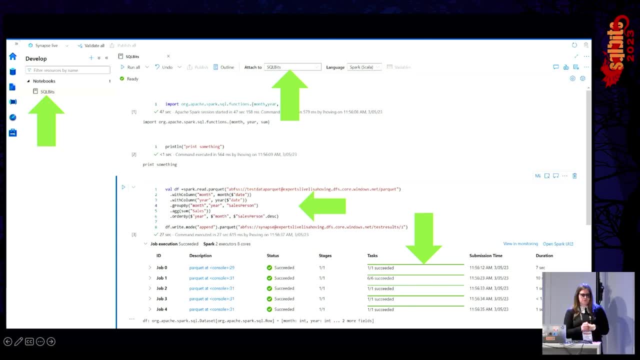 Okay, I read in the data, I do some aggregations, I add some columns And then I write it back to storage. On the last arrow below we can see all of the tasks And luckily for me, they succeeded, So I'm quite happy with that. 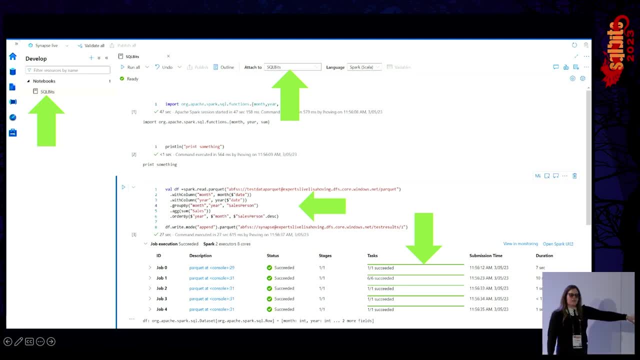 All right, But we kind of know the drill already. This is all cool and, all you know, quite a comprehensive platform, But why should we not use Synapse Analytics? As I mentioned, with Databricks it takes a lot of time. 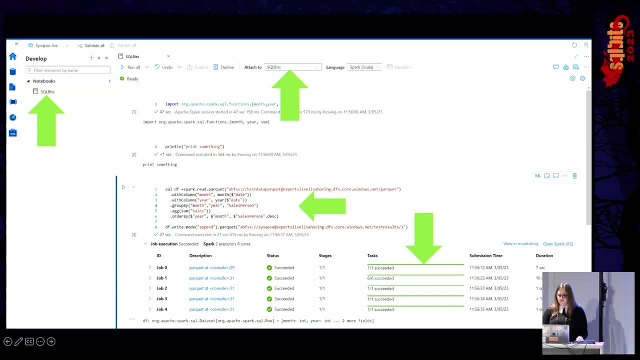 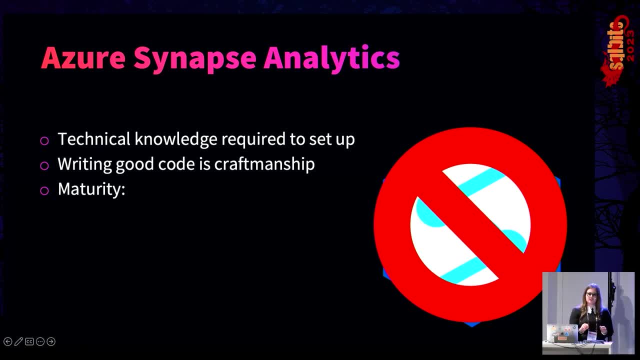 It takes a lot of effort. So quite a comprehensive platform, but why should we not use Synapse Analytics? As I mentioned, with Databricks, it takes technical knowledge to set this up right With all of these different things. there are all of these different aspects that we 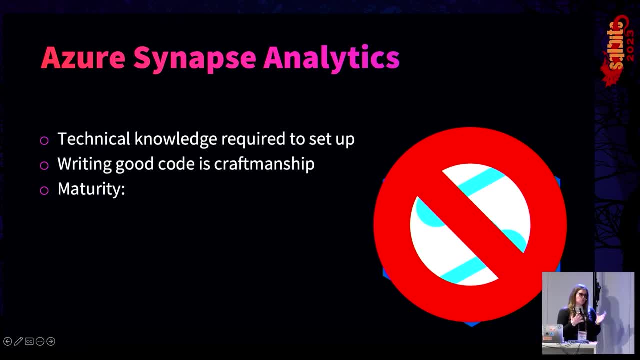 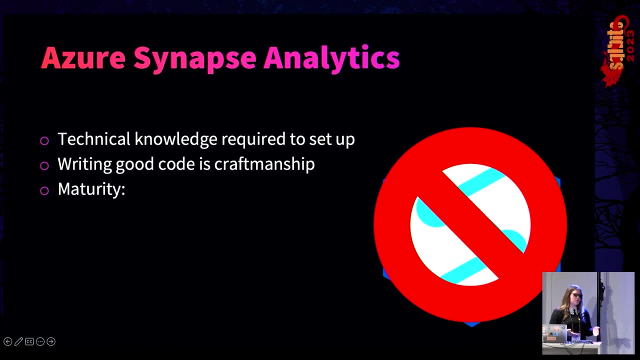 need to take care of when it comes to security, And that is super important. If you want to write code, whether it's KQL, Spark, Scala, whatever it's craftsmanship, We have to learn it in order to do it right. 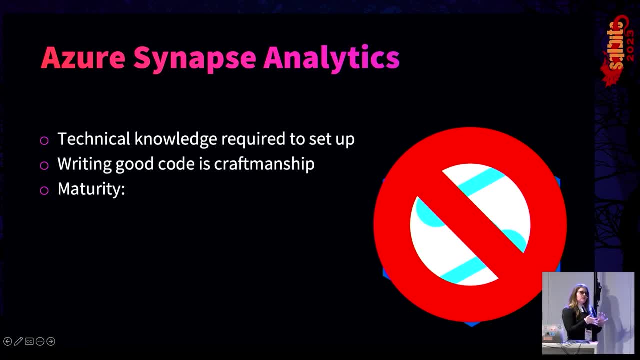 All right. And lastly, here is where it becomes a little bit more subjective. But in my opinion at least, the maturity of Synapse Analytics is not as great compared to Databricks yet, So I will show you why it's yet. 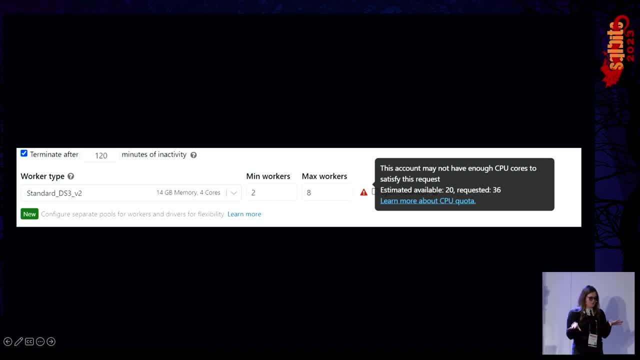 But just to give you an example, right? so I don't want to leave you here saying, oh yeah, it's not super mature, blah, blah, blah. Let's put it to the test. Let's have an example. 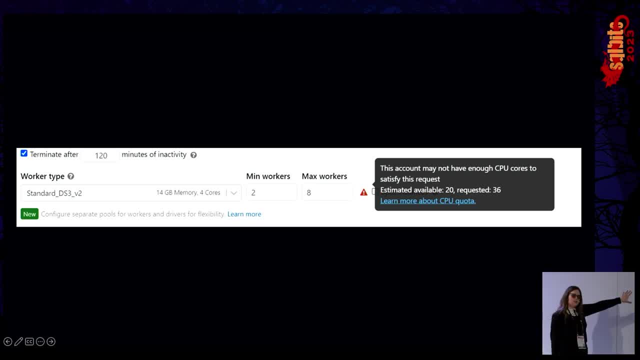 So this is an error that you would get In Databricks if you're using a subscription, because a subscription has, like, a maximum amount of virtual machines right. So if you have a subscription that is shared often, then you might run into this error. 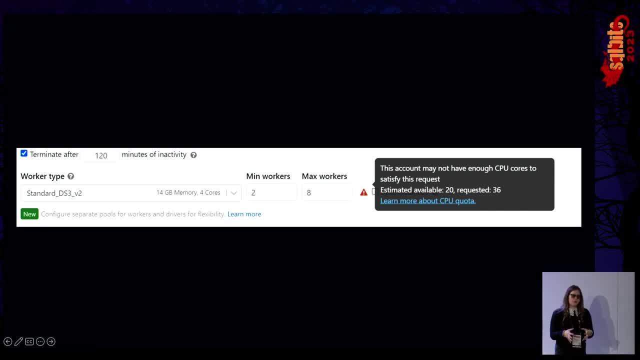 in Databricks. when you try to start to deploy that cluster, It might say: okay, well, Lisa, you could try to create this cluster if you wanted to, But if you do, you might not have enough cores to satisfy this request. 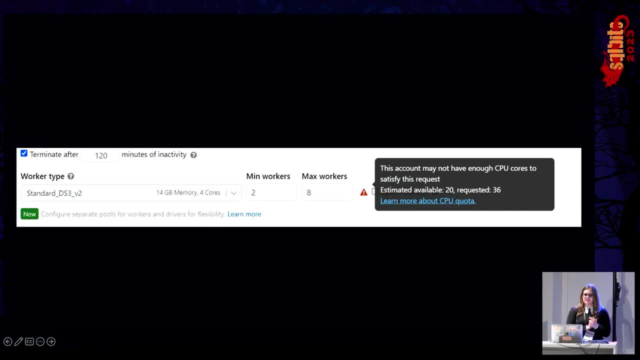 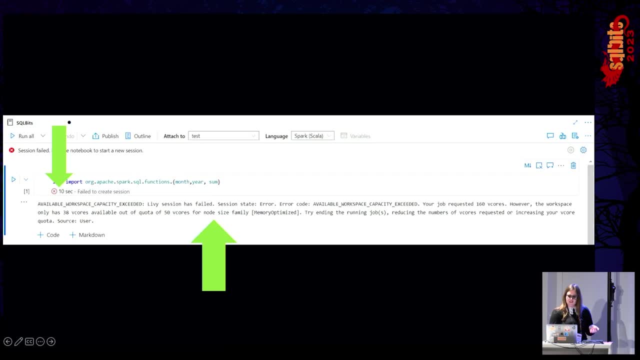 You can go ahead and start the cluster. I noticed that in the user. Yeah, I didn't have the right amount of cores And then it fails, But it gives me that error when I try to create the cluster. When it comes to Synapse Analytics, though, I don't get like any warnings. 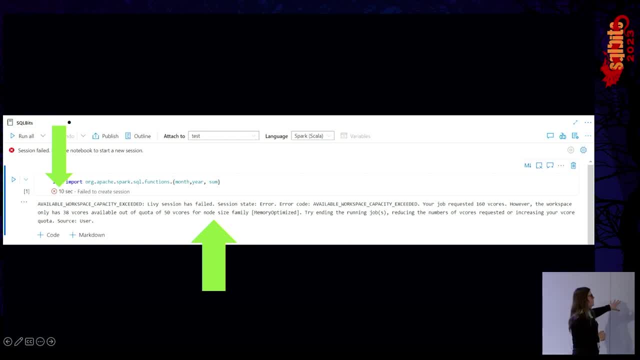 I just try to create the cluster And then I get this nice error: Available workspace capacity exceeded. Session has failed. I requested 38 vCores, which was quite a lot, So you know, But anyways, I got that error out right. 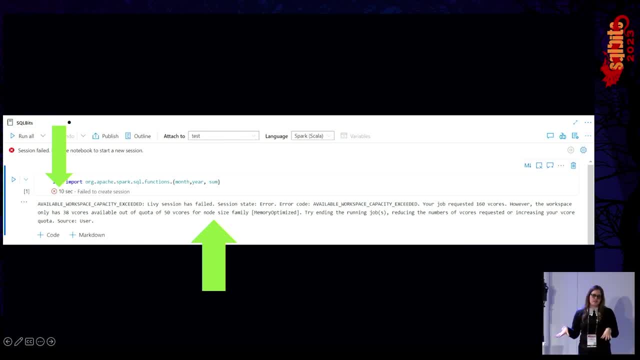 Out of that 50 vCores that I requested, I only had 38. So I took all of the time to try to spin up the cluster And then I got the error saying: oh, you don't have enough resource as well. 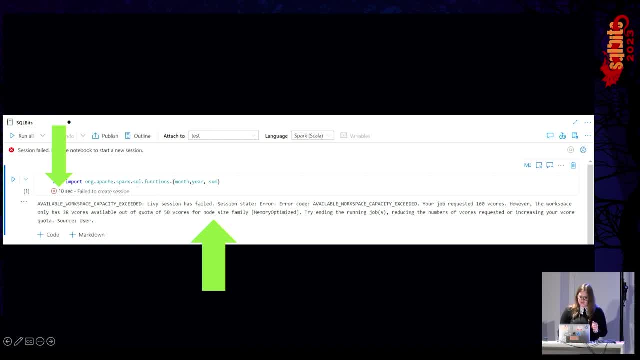 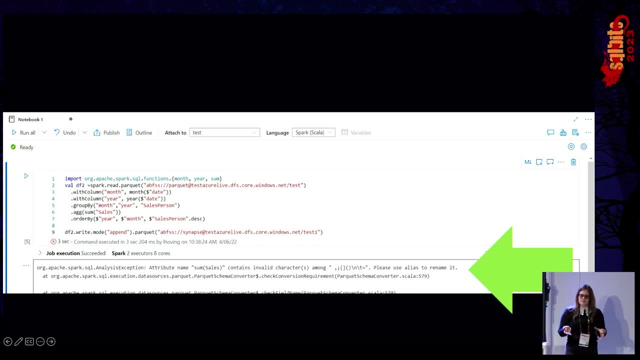 At that point, you know I'm pretty angry. But what happens with Synapse- and also with Databricks, of course- is that these platforms, they improve continuously. So one year ago I would have argued something else for Synapse Analytics. 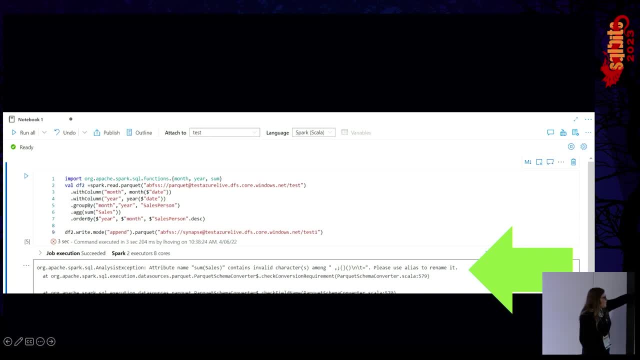 I would have said, hey, what I'm trying to do here to aggregate, that creates a column And that column by default has brackets, And I had run this in Databricks before. But when you try to save this in Synapse Analytics, I used to get an error saying, hey, these? 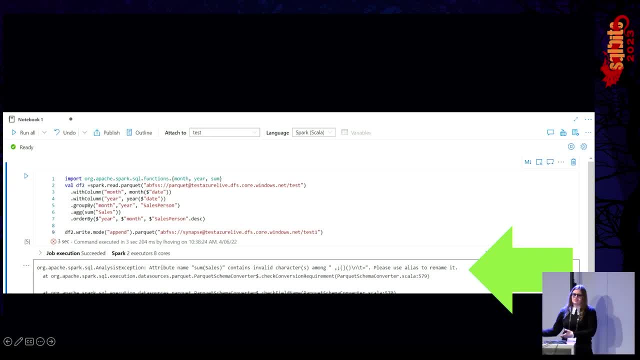 brackets that you have are invalid characters and hence you cannot save this back to your data lake storage. Pretty strange of an error, right? So I wanted to come here to SQL Bits to Wales and tell you all about this nasty little error that I got. 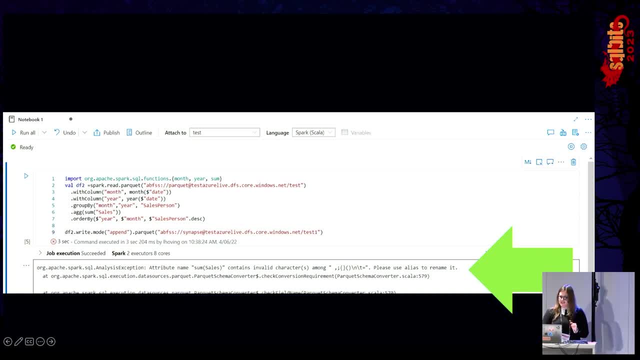 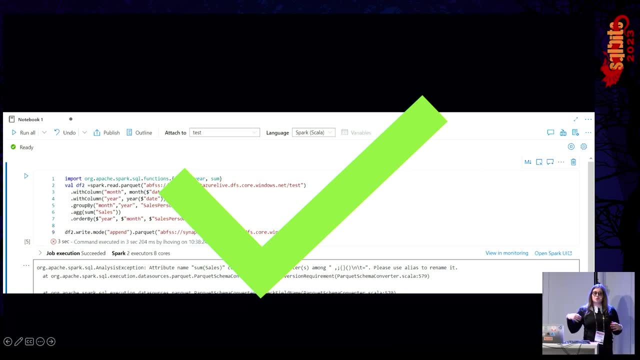 But I thought, okay, well, I tried to do it one more time, to run it, And then it passed. So just to keep in mind that these platforms they improve continuously, Time and time again. So every quarter they come out with really, really great improvements. 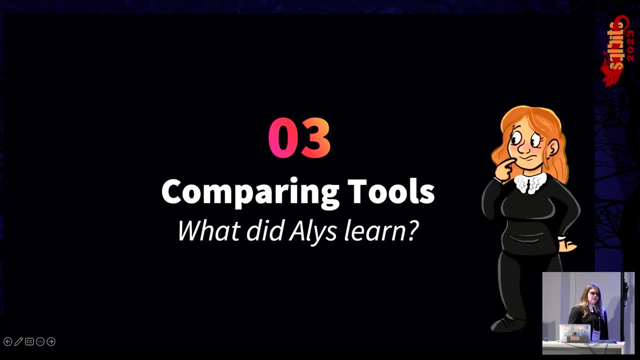 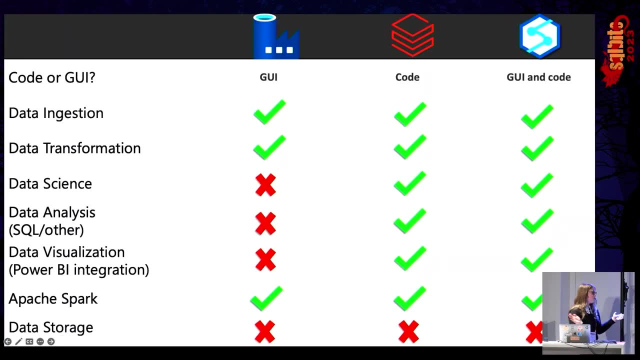 Okay, So let's compare these tools. Let's take a step back. What did Alice learn? So Azure Data Factory: you code using a graphical user interface drag and drop tool With Databricks and Synapse Analytics. we can write Spark, and Synapse is a little bit. 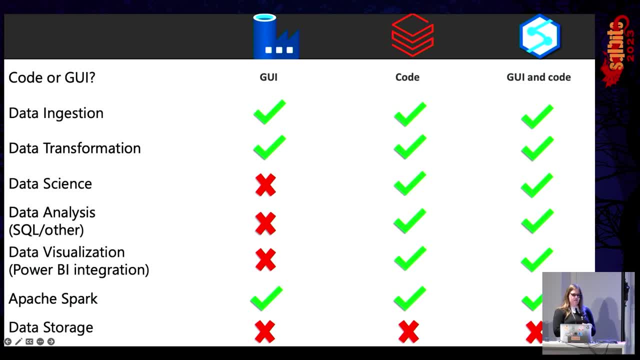 more comprehensive. It has that Azure Data Factory in it, right Synapse pipelines. When it comes to Azure Data Factory, you can do data ingestion and data transformation just fine. Okay When it comes to data science, data analysis and data visualization: Azure Data Factory. 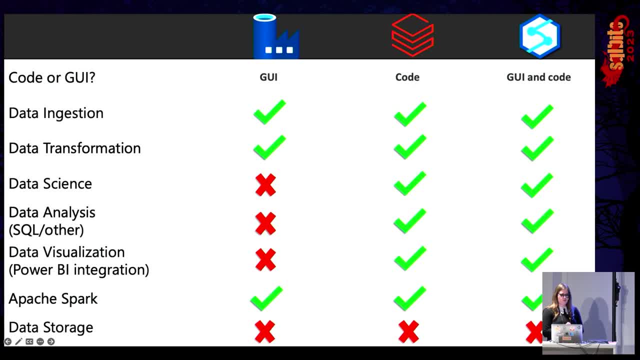 is not the tool for you. It's just not suitable for it. If you want to do Apache Spark, you can using these data flows and that power query. We're going to look at the cost a little bit later on. It's one thing good to know. 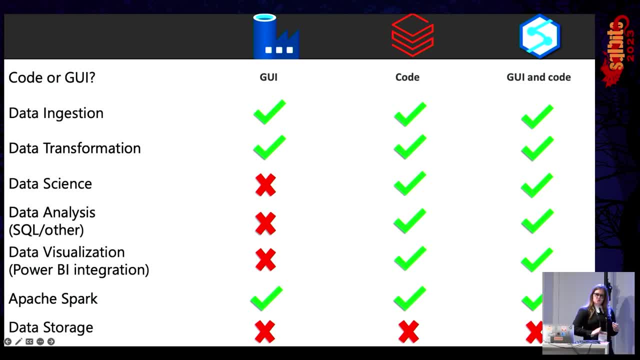 This is a question I often get from people. They're saying: Lisa, I want to store some data in Data Factory because it's a factory, right, I can store stuff in there. Well, no, Sadly no. And when you take it very strict, then you would also say that with Databricks and Synapse. 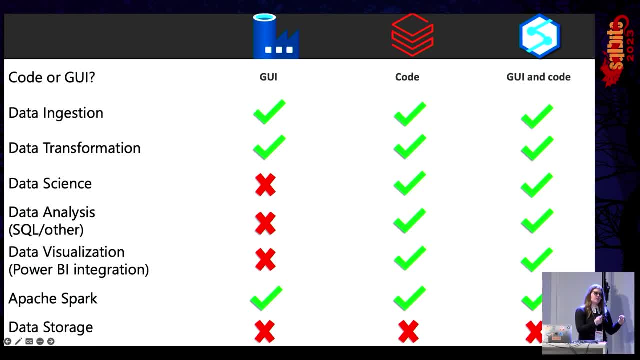 Analytics in the workspaces. we don't necessarily store data. We store that in our data lake, And that's something different to take into account. So we don't per se store data in any of these tools. But anyways, if you want to do data analysis, data science or even have this Power BI integration, 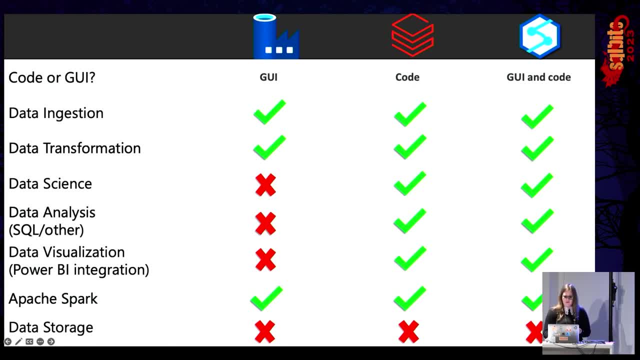 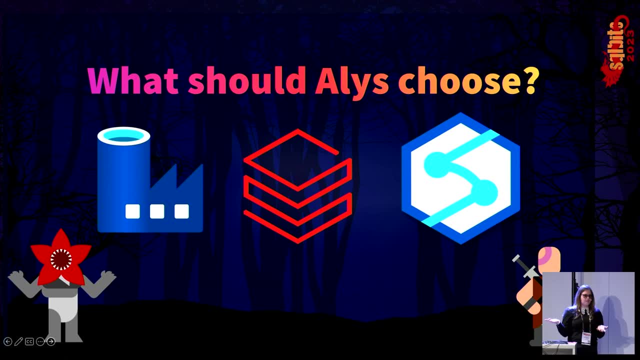 Databricks and Synapse Analytics are perfectly fine tools, So let me ask you again: What do you think Alice should choose? Azure Data Factory Databricks- I mean, I love Databricks, Synapse Analytics, All right. 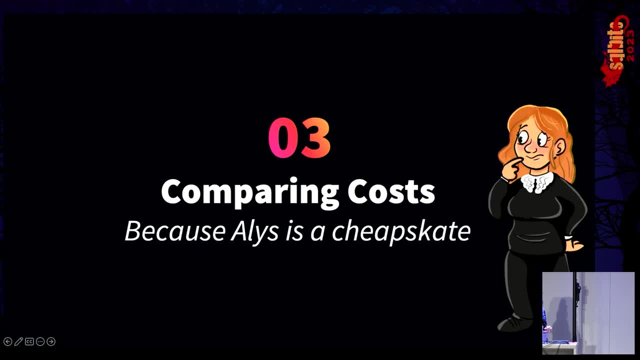 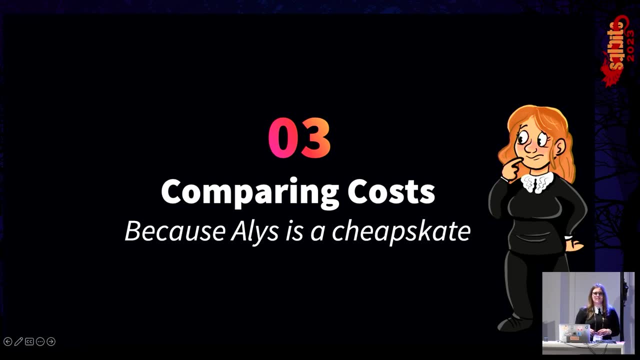 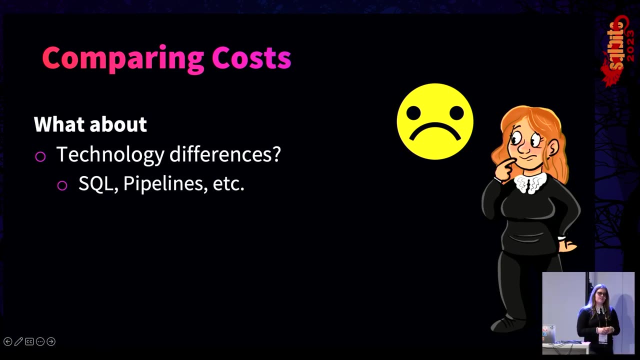 Interesting. Maybe we compare the tools a little bit more, Because, let's face it, We're all changing Cheap skates at some point, Want to have the most cost-effective tool. But is that really so easy? Can we just say, well, Synapse is the most expensive tool and Data Factory is the least? 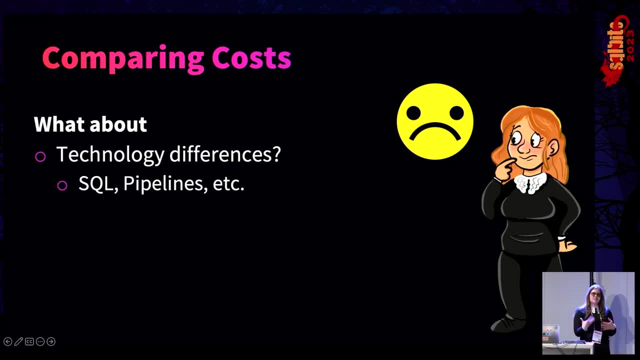 expensive tool. What about the technology differences? right, So Azure Data Factory has the integration runtime and the activities And we might have this use case using the SQL pools for Synapse And Spark for Databricks. Can we really easily compare these tools? 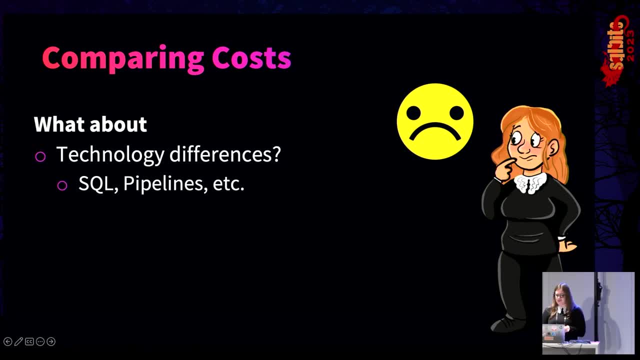 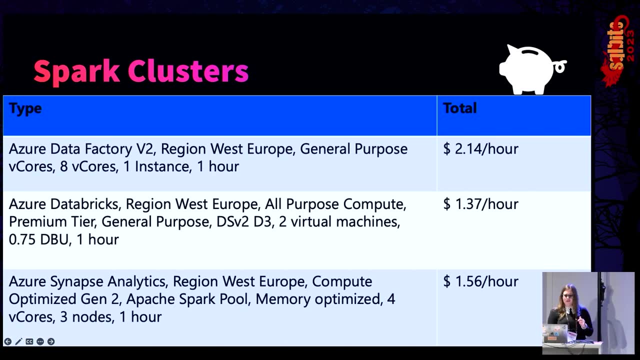 We would have to try out all of the use cases, right? It's just not that easily feasible, But I want to try, I really want to try. So I thought you know what All of these tools they use- Spark, right. 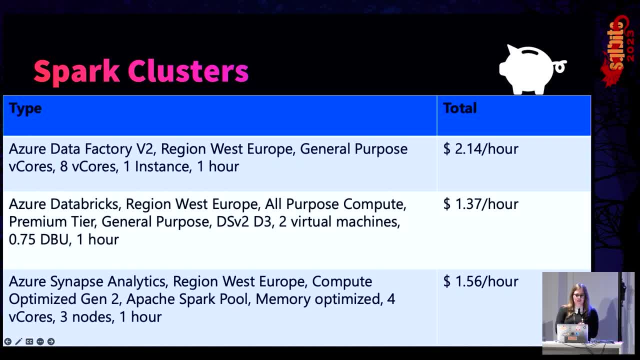 With Dataflows for Data Factory and Spark for Databricks and Synapse. So I tried to make three clusters that are, you know, comparable. So here you can see that Azure Data Factory is, you know, with these cluster configurations, a little bit more expensive than Databricks and Synapse Analytics. 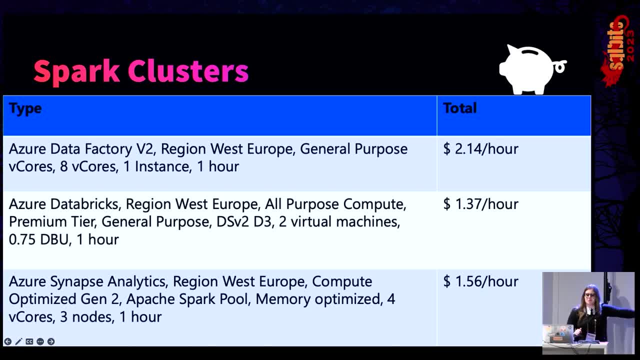 But in Synapse Analytics' favor. it's good to know that it has a little bit more computational power than Databricks has. if you look at this right, If you think I could do a better job, feel free to give me some feedback on it. 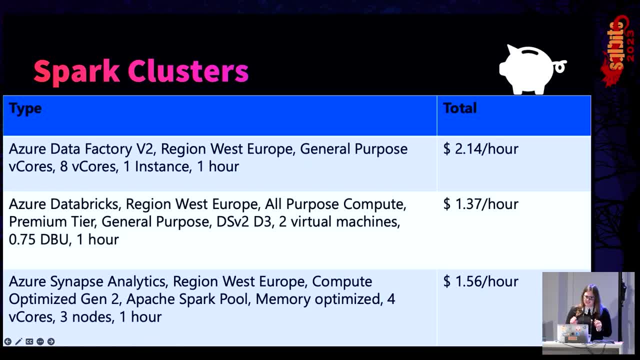 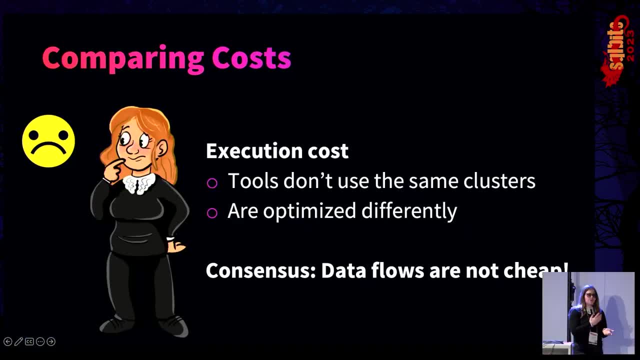 I would love to discuss this, because I think it's always, you know, difficult, But that's acceptable. That's exactly the point, Even if we could create three clusters that were 100% equal to one another, which we can't. 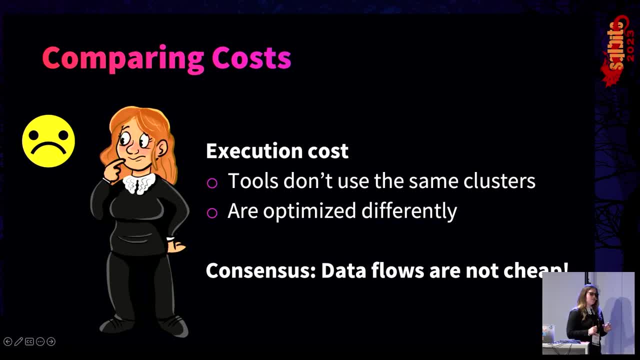 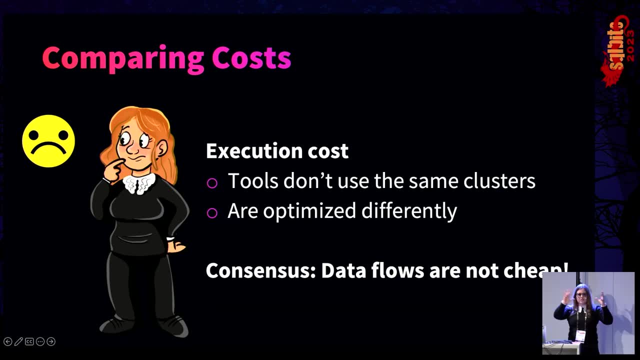 then we would find that these types of Spark that these tools use are optimized differently. So, Databricks and Synapse Analytics, they put their own, let's say, sauce over it and they optimize Spark. So the Spark that you download from the Apache Spark website is not the same as the thing. 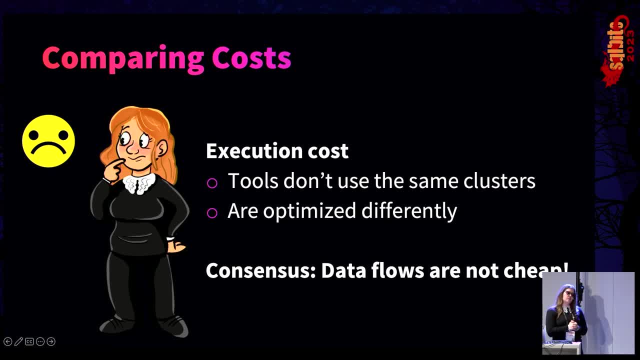 that you run in these tools. It's good to keep that in mind. But if you are so inclined to make a decision based on cost, then it is good to know that data flows in general, at least in my experience. so Azure Data Factory with Spark is not cheap. 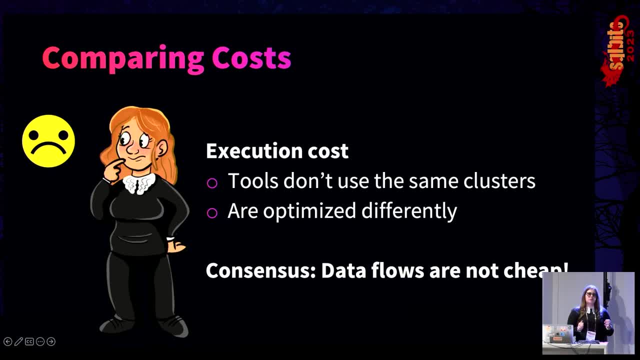 So that's basically what we find is that if we migrate our workflows from Data Factory data flow, so using that Spark, to, let's say, programming Spark ourselves, then that you'll usually, you know, we gain a little bit of money. 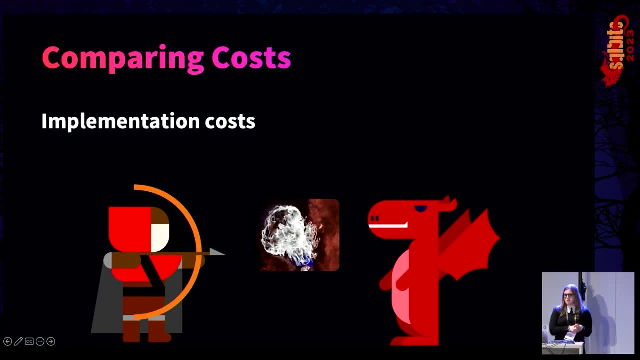 One thing on costs, of course, that we always have to mention is the implementation. cost is maybe a bit implicit, But if you're used to using Databricks, go with Databricks, Don't you know, start implementing Data Factory or whatnot? 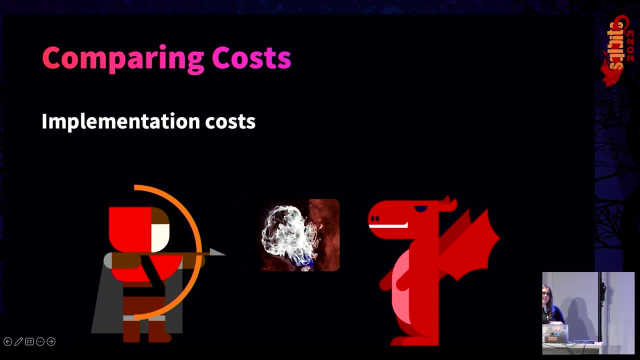 And we actually have quite a lot of customers that do this. You know, you hear like a great talk from somebody think, oh, Synapse Analytics is the latest and greatest thing Let's all migrate to. you know, Synapse Analytics. 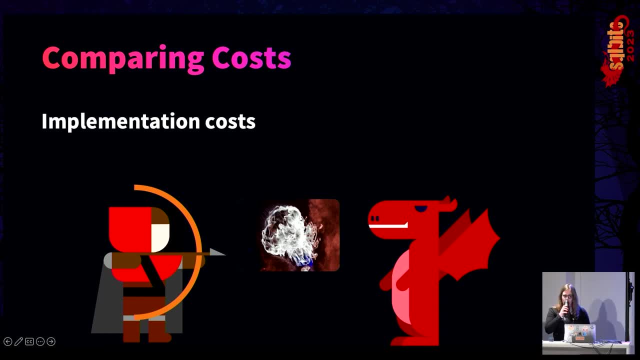 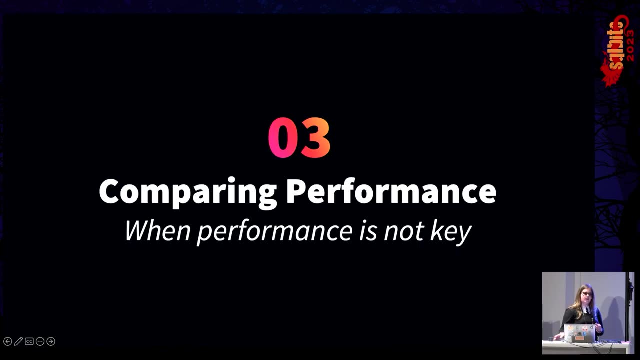 But you know that comes at its own cost. Okay, Let's start thinking: If I cannot have the cheapest tool, then just give me the one that performs best. right, Because I don't like waiting, And performance is usually key here. 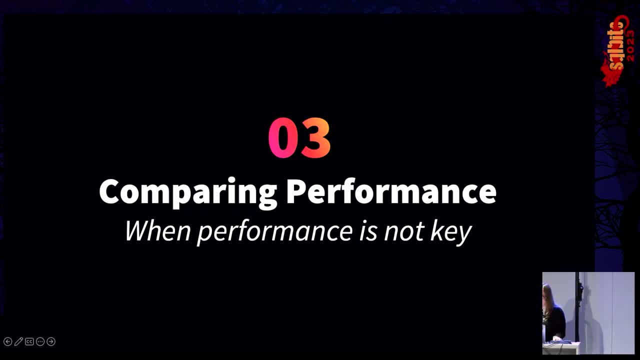 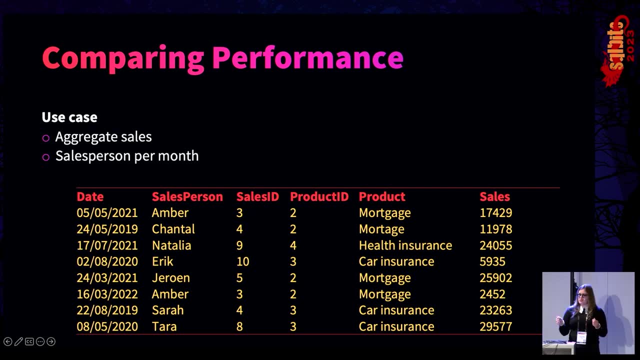 So just give me the tool that performs the best, Fine, So let's think about this, Think about that. So can we really compare these tools based on performance? At least I want to try. So I implemented Alice's use case for all of these free tools. 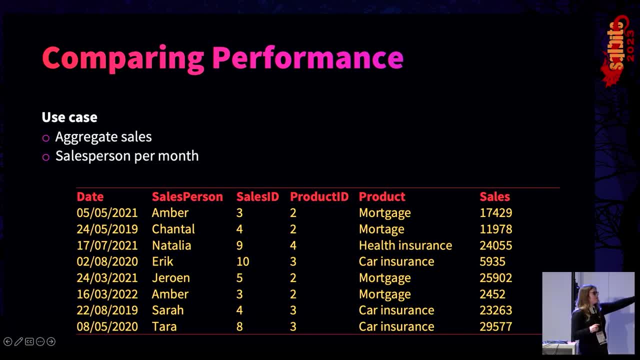 And just to give you a quick recap on her use case, she wanted to aggregate sales on salesperson per month to see what person outperformed throughout the month. So I ran this in all these free tools three times. I mean that's fair right. 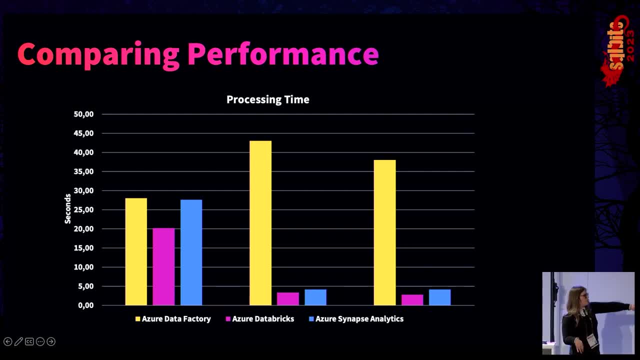 So the first, If people are color blind, the first thing is for Data Factory, then the second thing is for Databricks and then the third one is for Synapse Analytics, because I don't know how inclusive these colors are. Probably not. 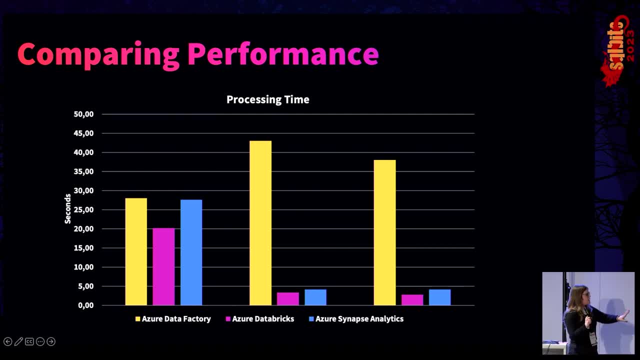 So what we basically see here? the first thing that comes to mind is that Azure Data Factory- they don't cache their results, So every run is going to be about equal amount of time. Databricks and Synapse Analytics. however, in Spark they do cache results. 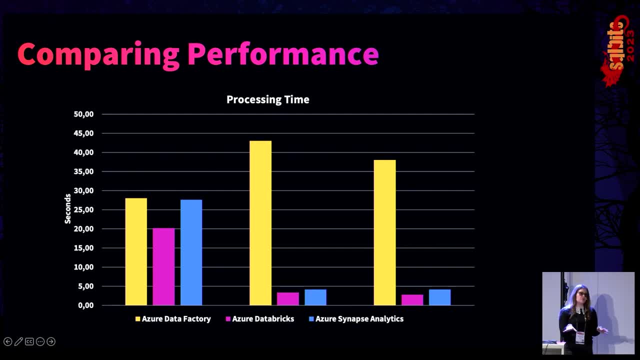 So the second and the third run that you get is immediately good. They're going to be a lot faster, a lot quicker, So it's good to take that into account. But I want to know the cost. So if you look at these cluster costs that we just looked at, how expensive are these? 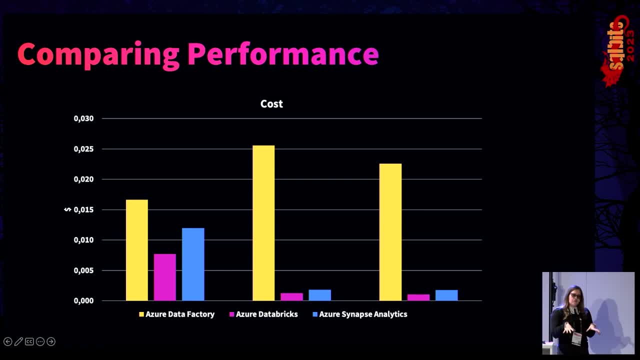 runs going to be. So what we see for Alice's use case is that, as expected, Azure Data Factory is not the cheapest tool. Actually, Databricks is For all of the three runs. I would say Databricks comes first on performance. 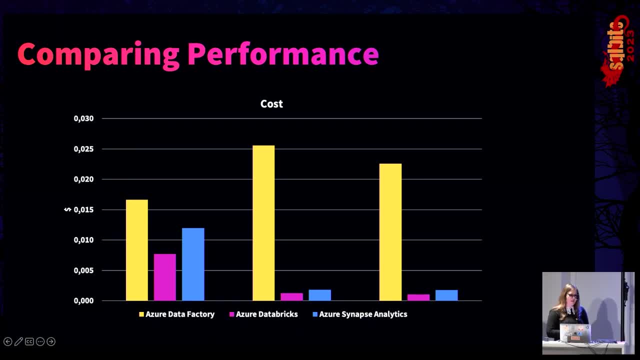 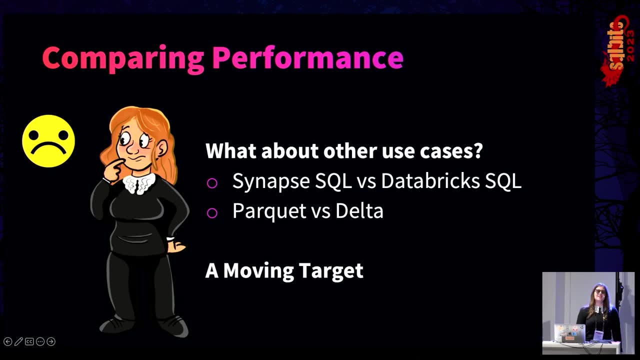 Performance and costs, then Synapse Analytics and then Azure Data Factory. But let's take a step back. Is it really so easy to just conclude? well, this use case. you know Databricks performed best. Just go with Databricks. 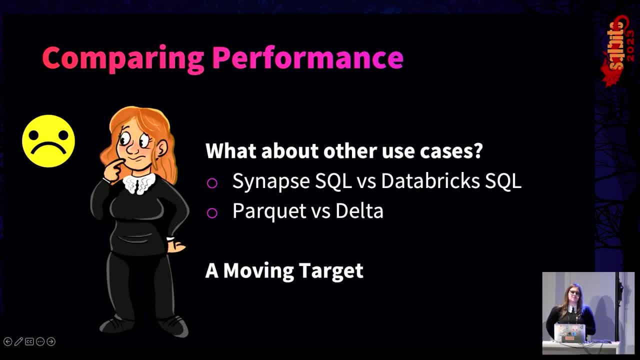 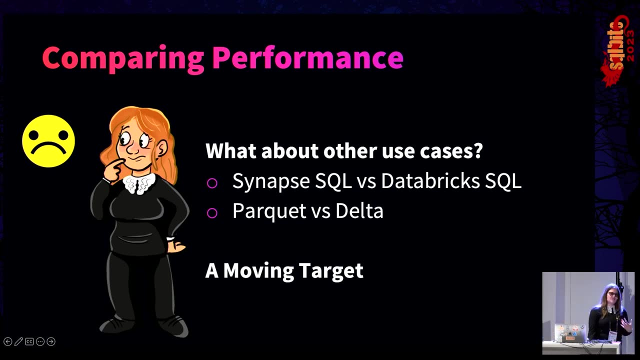 What about other use cases? What if I had implemented this using SQL versus Databricks? SQL, You know Shiny photon engine. What if I had stored these results in delta instead of parquet? These performance differences then still be the same. 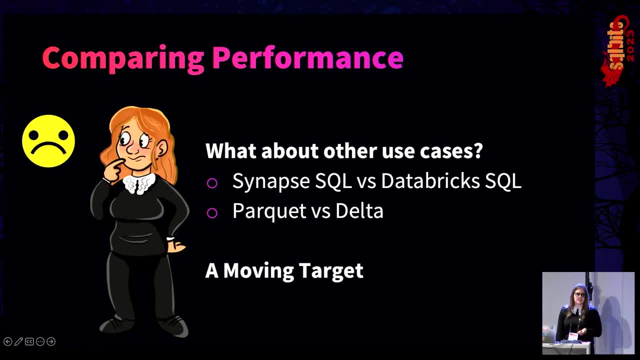 Probably not right. Maybe in that case Synapse Analytics would have performed best and would be the cheapest tool. Do we really want to make a decision on what tool is best based on just one use case? And even if we wanted to do that, 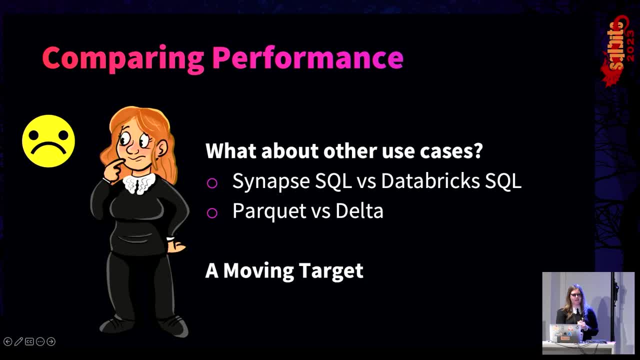 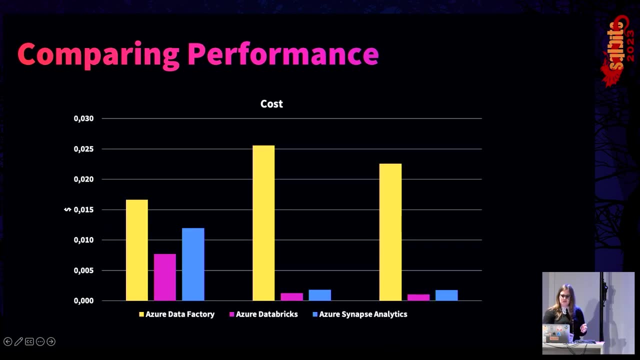 And we start implementing. And we start implementing, let's say, Databricks today. how is the performance going to be tomorrow? Because, as I mentioned, all of these tools, they come out with new functionality every quarter, So maybe next quarter everything is going to be different and that's also why these 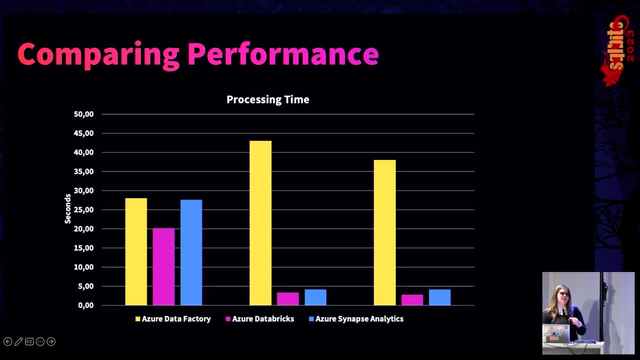 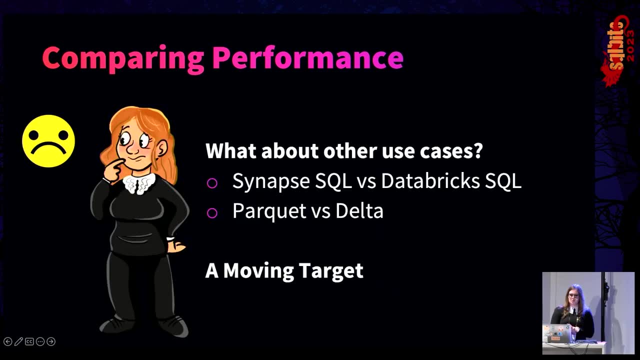 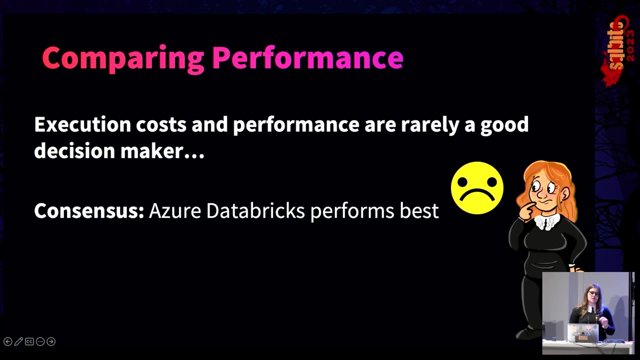 kind of benchmarks that I do. I rerun them every time that I do a new talk and every time I get different results. That's quite interesting, right? That moving target? All right, All right. So in the end I would say execution costs and performance. they are rarely a good decision. 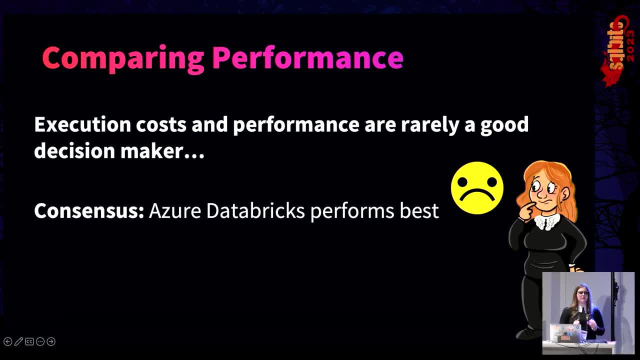 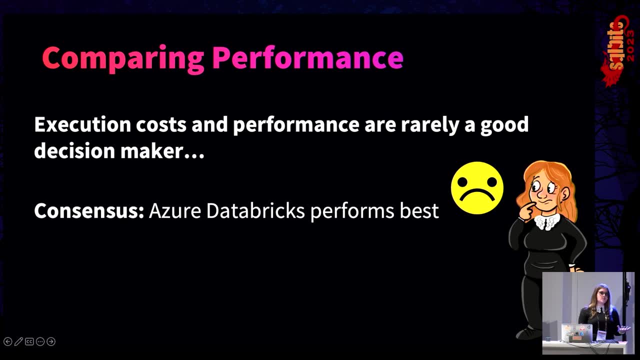 maker. But if you are so inclined to make a decision based on cost or based on performance, then I would say that consensus, at this moment at least, seems to be that Azure Databricks performs best. You also see it in other people's benchmarks. 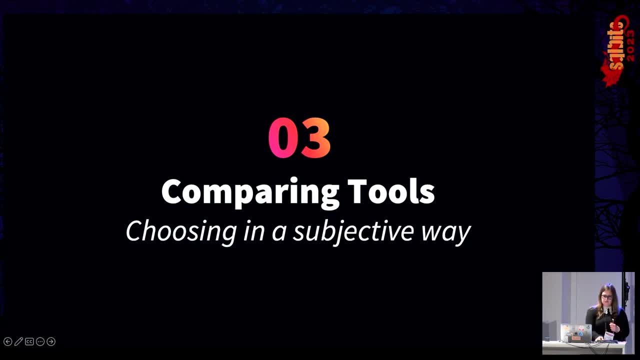 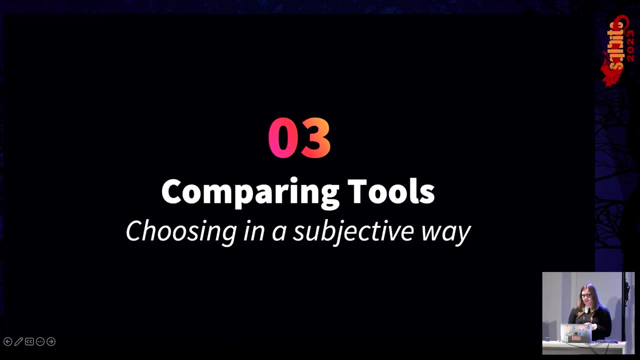 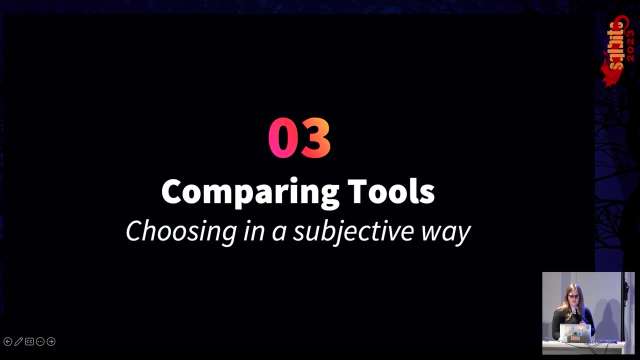 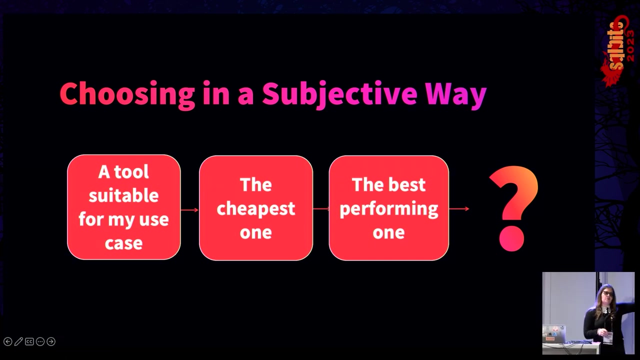 All right. So all right, What are we left off with? Alice starts thinking, Can we maybe make a decision in more of a subjective manner? So Alice first thought: I want to have a tool that is suitable for my use case right. 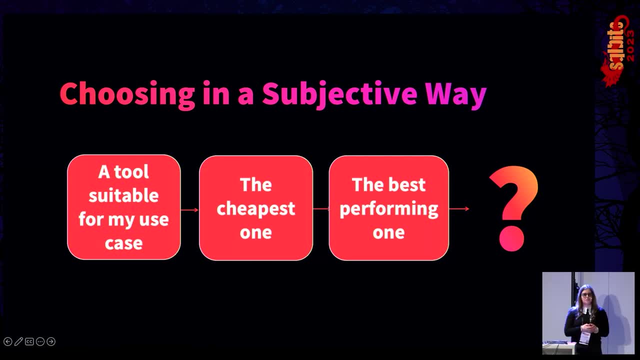 And then we found that Alice had a use case for data aggregation, Maybe sorting a bit So she could use Azure Data Factory, Azure Synapse Analytics and Azure Databricks just fine. So then she thought, well, if I can do all of these use cases with all of these tools. 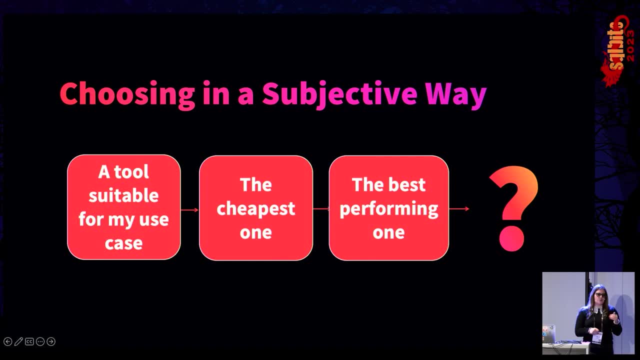 just give me the cheapest one right to run. But then, well, we could see what was the cheapest tool for Alice's use case, but we didn't really know if that would work for all of the use cases, So that didn't really, you know, work. 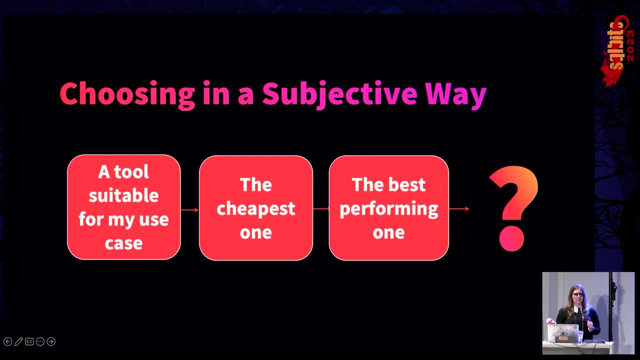 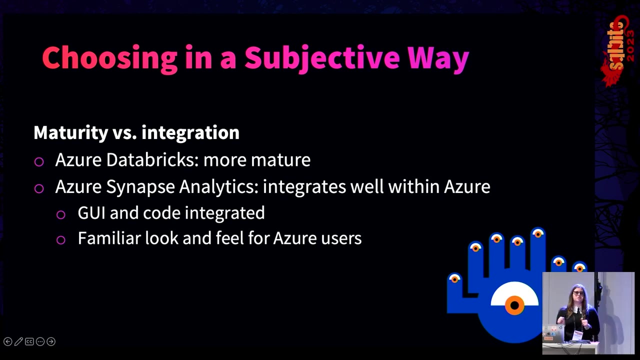 So she thought, just give me the best performing one. But then we kind of ran into the same issue. So let's make a decision in more of a subjective way. In my opinion, usually it's a maturity versus integration question, And that's subjective right. 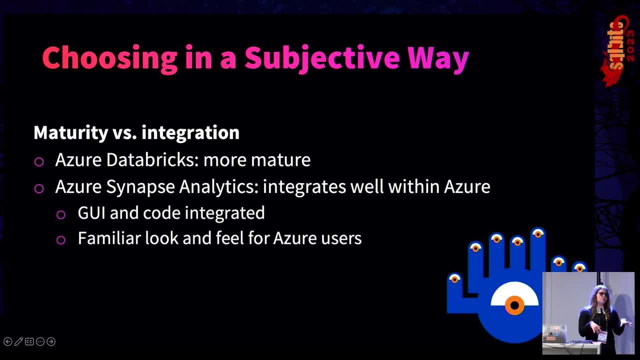 So, in my opinion, as we saw, Databricks is a little bit more of a mature platform. So people that start using it, they get acquainted with it a little bit easier, And the things that you run into the nitty-gritty details of things, you know, that's just. 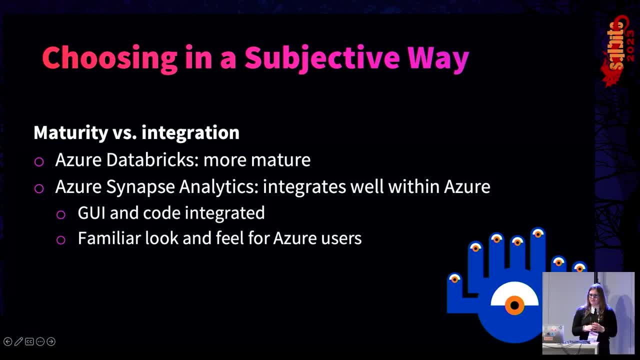 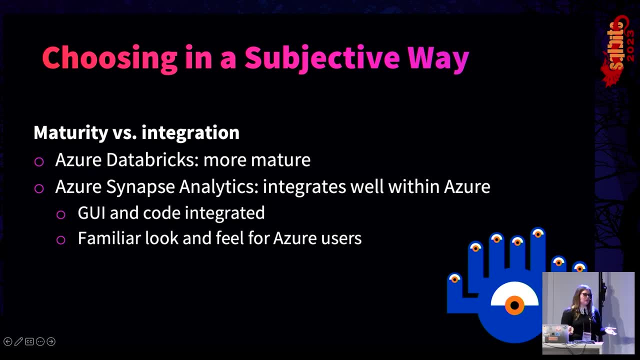 a little bit less with Databricks It goes a little bit smoother. But I mean Azure Synapse Analytics is like Unity. It integrates super well within the Azure platform. It gets all of these new shiny tools, The graphical user interface, from the Synapse pipelines. you know that's integrated with. 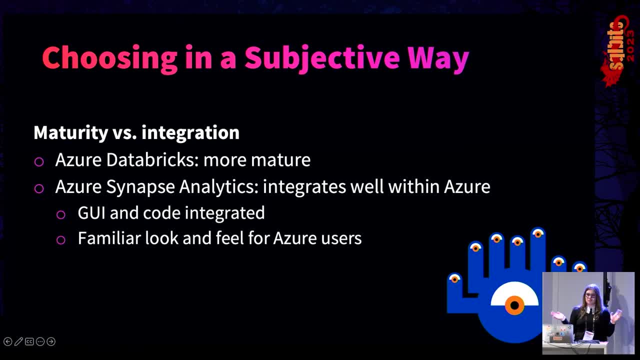 code. So we have Azure Data Factory, basically in Synapse Analytics, which is pretty cool. And if you are familiar with the Synapse Analytics, you know you're probably familiar with the Azure Data Factory And if you are familiar with the Azure platform, then you will find the Synapse Analytics a. 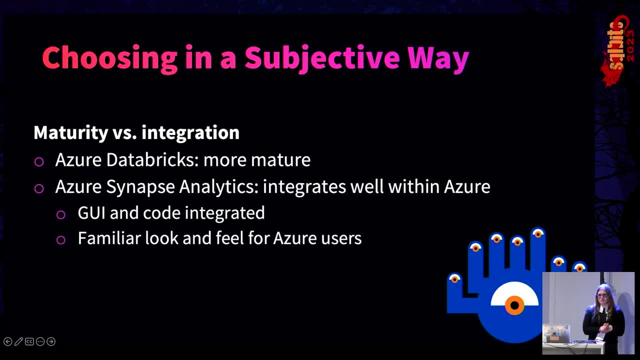 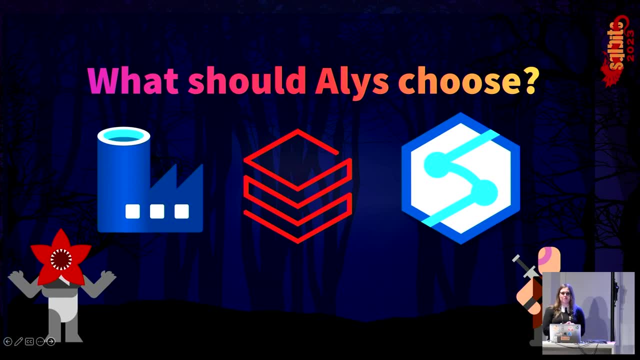 platform that you're pretty much already acquainted with, So that's pretty cool too. So what do you guys think Alice should choose? Who thinks now Azure Data Factory- All right, I mean, there are basically no wrong answers here- Databricks. 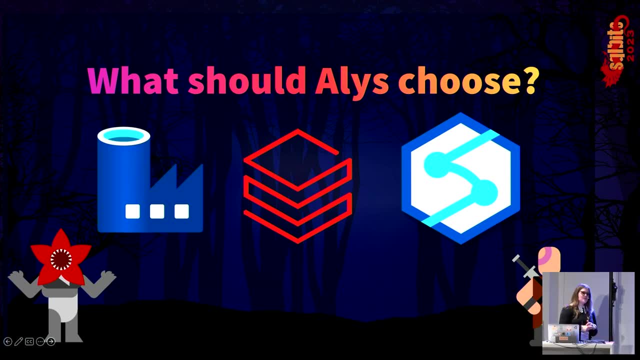 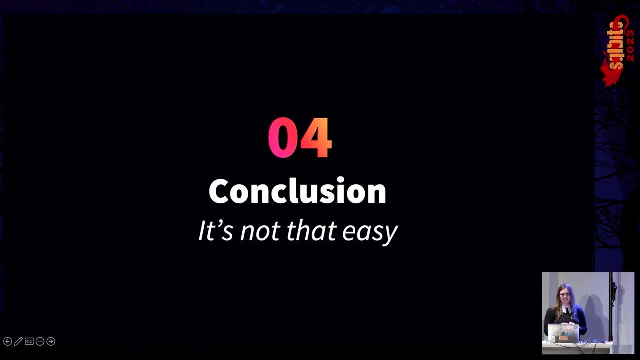 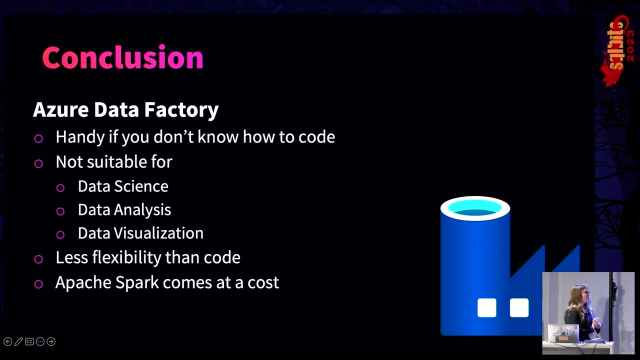 I love Databricks too. Synapse Analytics: All right, It's not that easy, Yeah. So Azure Data Factory: right. that tool comes in handy for people that don't know how to code, If you don't know how to code and you need some data integration, so ingestion or transformation. 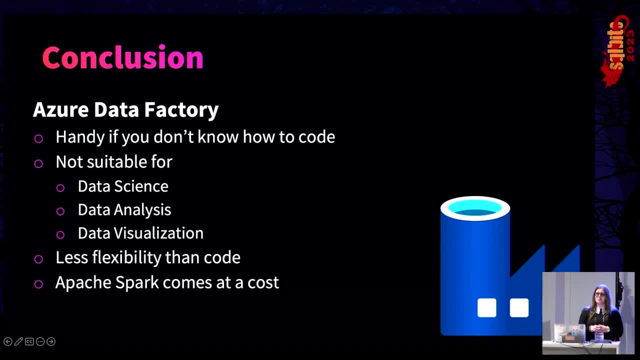 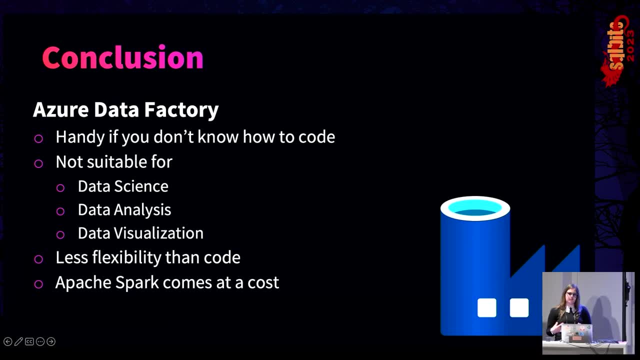 then use Azure Data Factory. I see a lot of customers implementing this with no experience on how to code, and this works perfectly fine for them. However, if you want to do data science or data analysis, use cases, if you want to do visualization, and, for the love of God, don't store data in Data Factory. it's not possible. 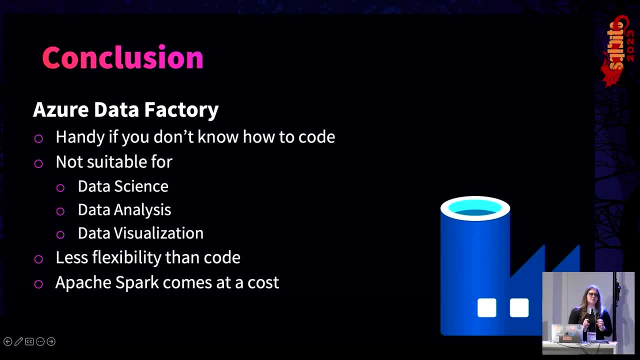 but then it's not the tool for you. It does offer us a little bit less flexibility than code. You know we cannot reuse all of these functions that we have And if we want to run that cool Apache Spark, you know, in the Power Query or in the data. 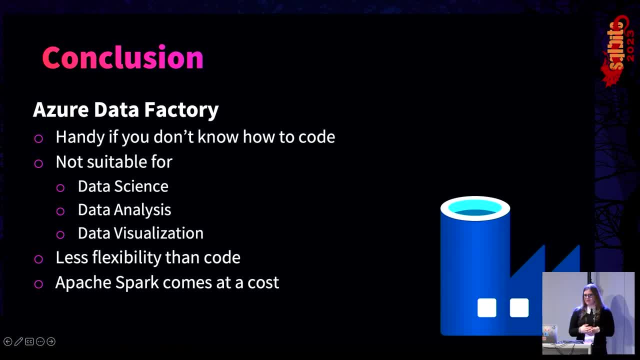 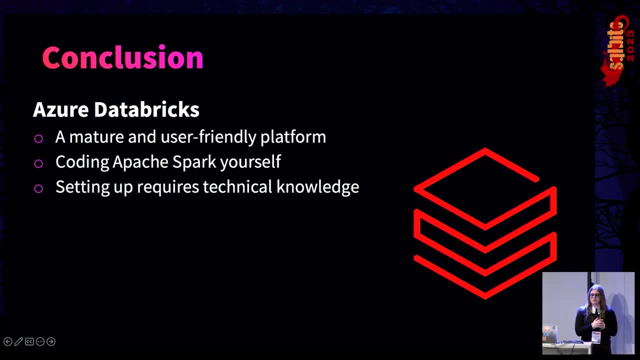 flows, that does come at a premium, usually speaking, When it comes to Databricks, we get quite a mature and user-friendly platform. People that start off with Databricks are usually quite content and happy with it, But do make sure that you know that coding, Apache, Spark yourself- you know that's craftsmanship. 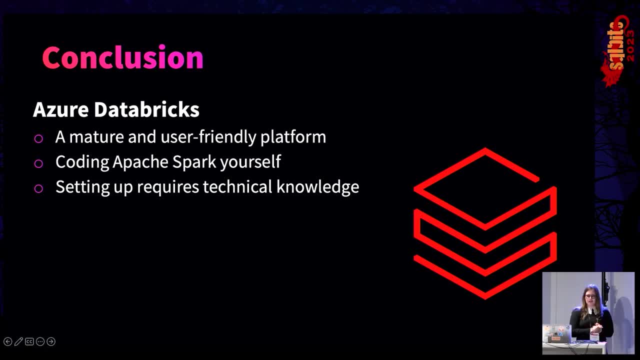 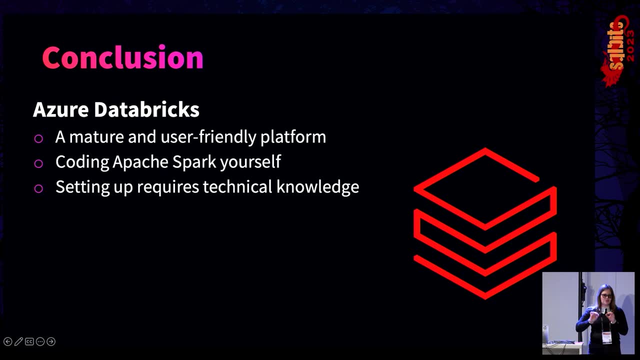 Setting up Databricks, Not just with Synapse Analytics, but arguably also with Data Factory. It takes technical knowledge to set it up right, But especially Databricks and Synapse Analytics. as you saw, if you don't do it right, you're. 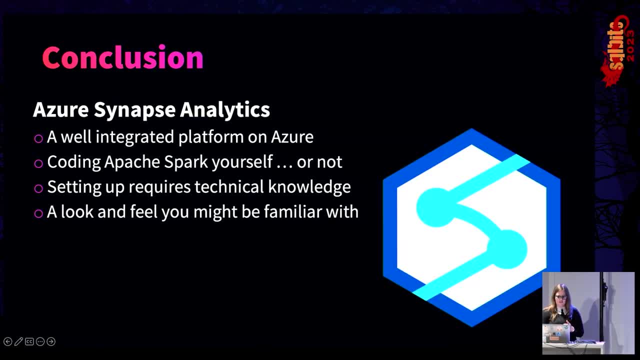 going to have some trouble. Synapse Analytics, however, offers us a well-integrated platform. on Azure We get all of these great, shiny new tools. If you want to code Apache Spark by yourself, That's totally fine. You know, we can do NET, we can do Scala, we can do Python, whatever. 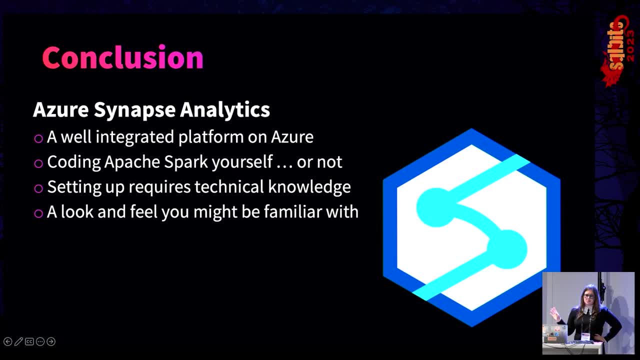 But if we don't want to code, then of course we still have these Synapse pipelines, So that's pretty cool. As I mentioned setting it up, I'll just repeat it again: It takes technical knowledge, so please do your research. 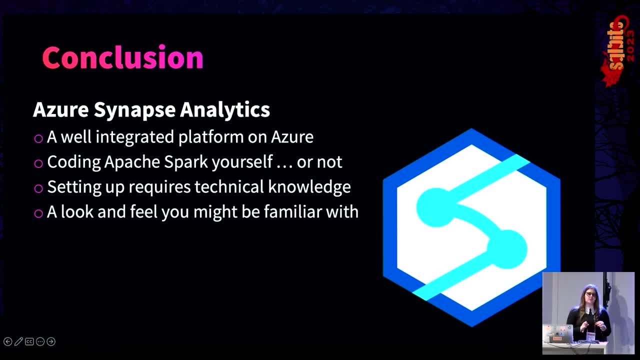 But if you do your research right, you will find a look and feel that you might be familiar with, if you know the Azure platform, And exactly for this. So, for this reason, I would probably advise Alice to go with Azure Synapse Analytics. 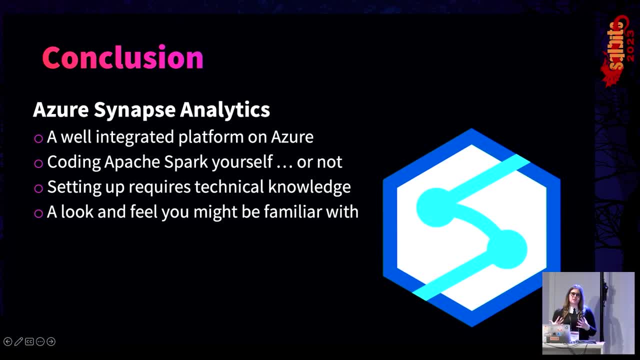 Because she has some coding experience. So if she doesn't want to pay a premium for the data flows, then she can code Apache Spark herself. She can give that a try if she wants to. Well, if you then look at Synapse Analytics or Databricks, given that she's already acquainted, 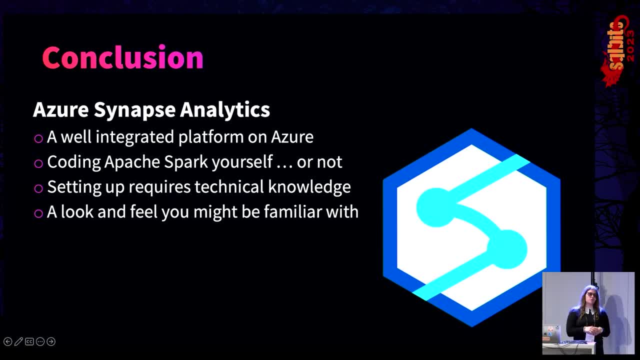 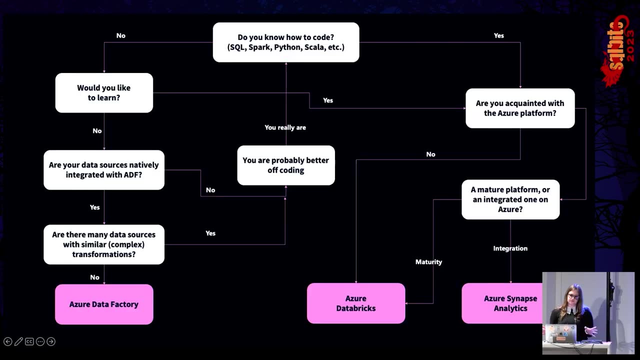 with the Azure platform. in that case, I would advise her to go with Synapse Analytics. If that wasn't the case and she was a little bit more new to the Azure platform, then she would say: go with Azure Databricks because it's a little bit more mature overall. 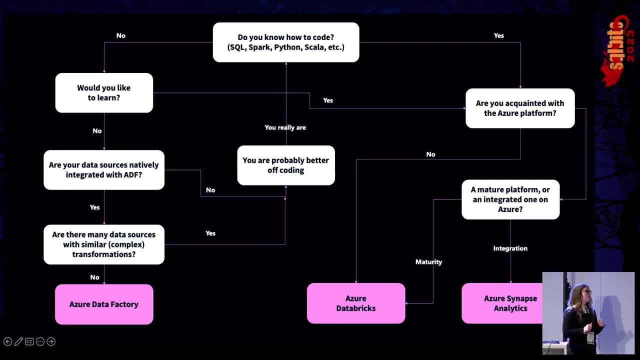 So, okay, I have a little chart to make a decision. So if you don't know how to code and you don't want to learn boo, then question yourself: Are your data sources natively integrated within Azure Data Factory? If they are not, you are better off coding. 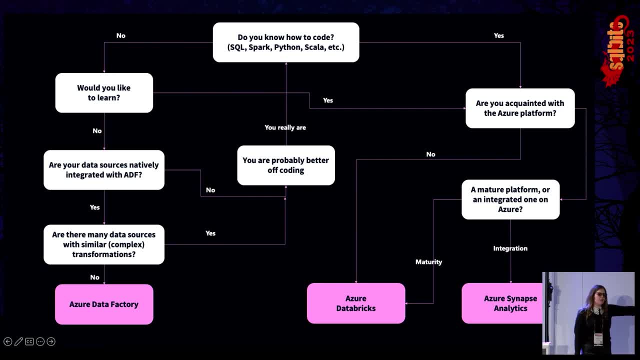 Trust me. But if they are, think about it. Do you have many activities, many pipelines to create? Do you want them to be made in a generic way? Then probably think about coding again. But if this is not the case, then you know, feel free to go with Azure Data Factory.